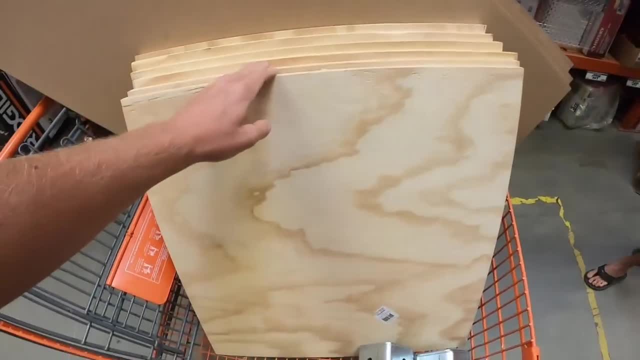 But I'm going to have to cut these a little bit smaller Guys. so I have these small pieces of plywood. Here's some metal. This one's pretty thick and I found this medium density thick stuff. I think it's super strong. 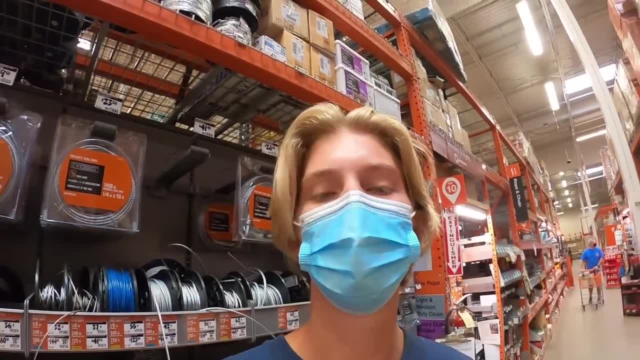 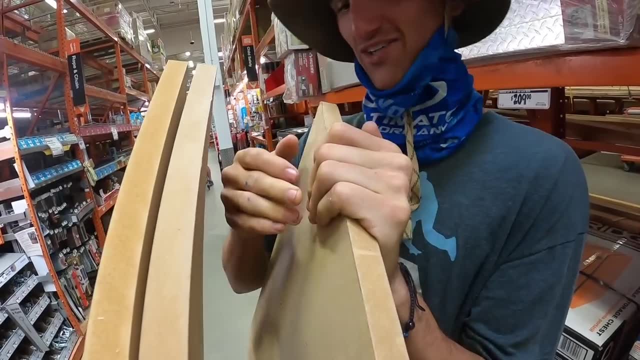 And we're just going to try to reinforce it with metal brackets and as many strong materials as possible. You think this is strong, Just kidding, Eat it. Okay, it's strong, Okay, good, And then I'm going to put a safe in it. 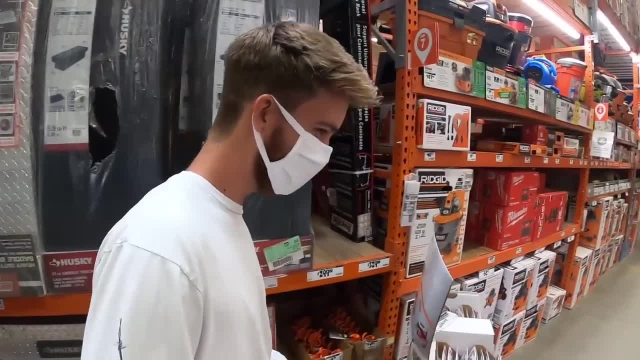 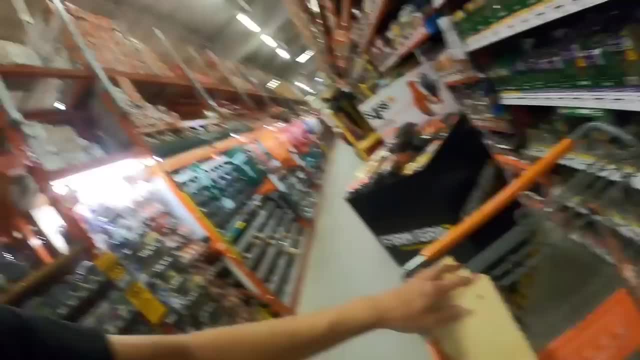 Wait, let me punch it Because you know I'm going to put a safe inside my unbreakable box. We broke it into safes before just saying Good luck. So recap on my items: I'm going to be using 2x4s and plywood for the structure of it. 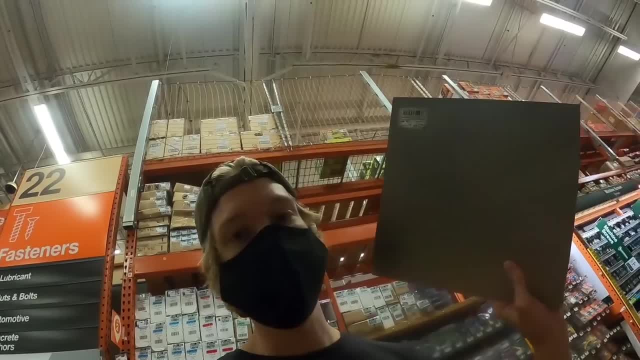 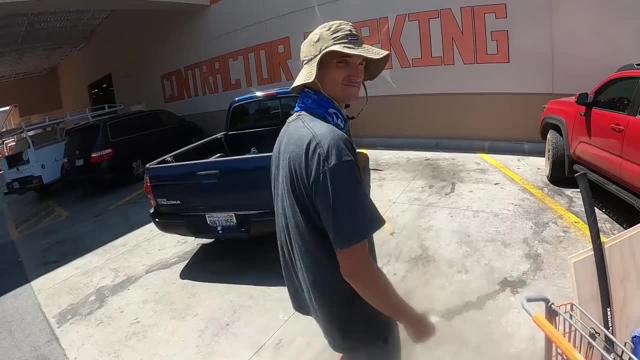 And then after that, I bought these metal plates which I'm going to be bolting in. Then I have these brackets I'm going to be bolting onto the sides and the corners. Ryan, whose box do you think is going to be stronger? 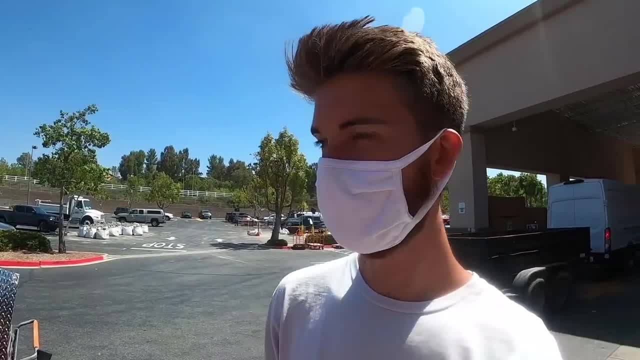 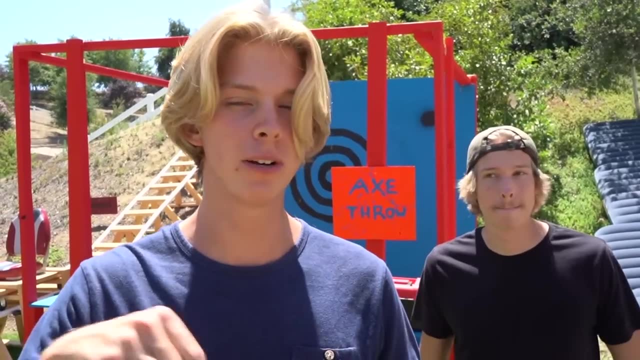 Probably Rob's. Jeff just dropped his nuts. Jeff just dropped his nuts. We are back home with all of our supplies. Now we need to determine whose phone goes in whose box, Because you got to put your phone in someone else's box. 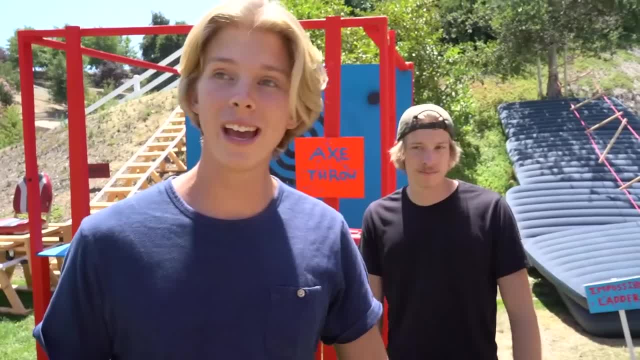 And then you break into the box with your phone, And if you can't get your phone then the box is dumped into the trailer. And guess what That thing is going to dump? So your phone is gone, You have to buy a new one. 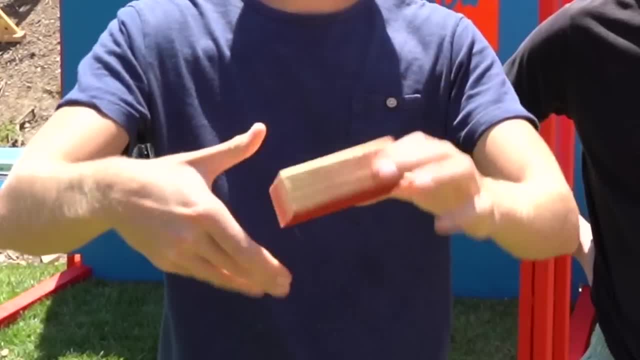 So I'm going to throw this block. If the red is up, we'll pass the phones to the left. If it goes without red up, you pass to the right. Right, Are you ready? Yep, Everyone get their phones out. 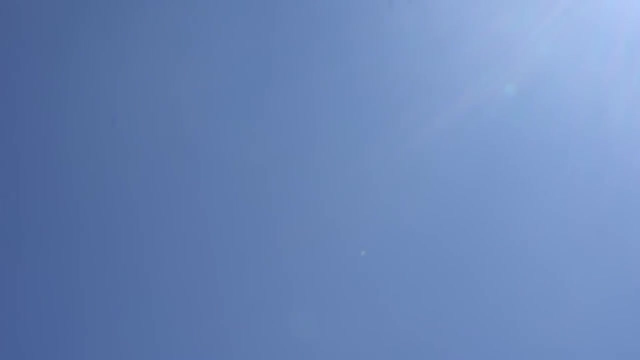 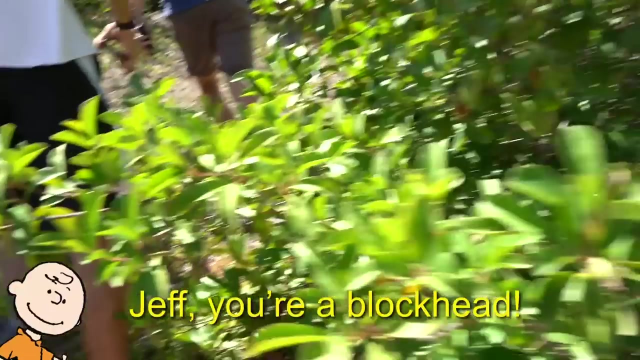 Here's my phone. Okay, I'm going to flip the block. Are you ready? Flip the tag. Where is it? Oh, it's over here. Where did it go? Look what you did. You lost the block Because you're a block head. 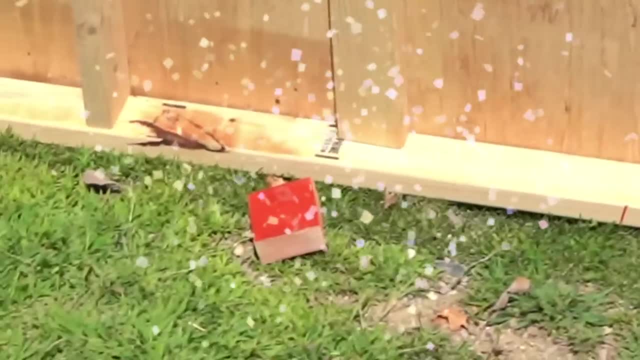 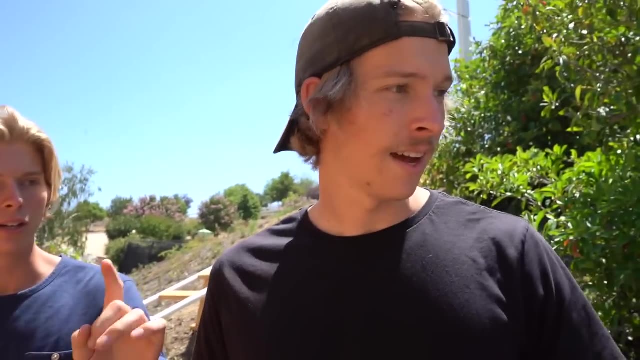 I think it's in this, bush, It's red. What? Pass it to the left. No, Oh, You're right, It's right. here, It's really red, You're right. Okay, So we have to pass it to the left. 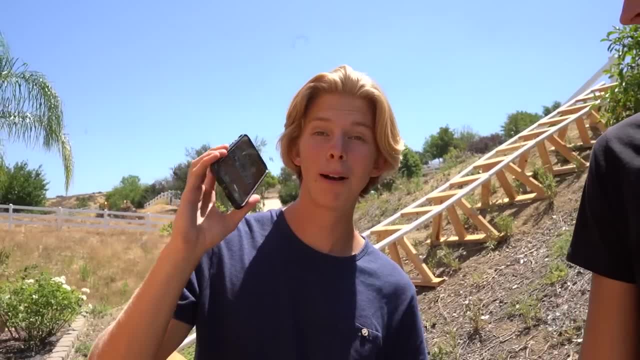 So, Robert, you get my phone, Chris gets my phone And Chris Jeff's phone. Chris' phone. Jeff gets Chris' phone. Chris is going to break my box. Rob is going to break, Chris is. No, I'm going to break Rob's box. 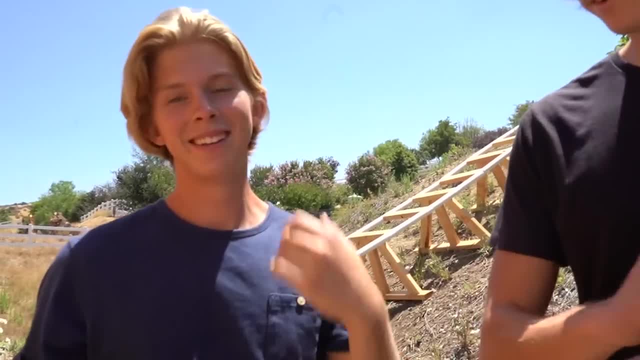 I'm breaking Chris' box Right. This is confusing. No, no, no, They get it, They get it, They get it. Let's get buildy. Okay, So first we need to bubble wrap Chris' phone in some very thick wrap. 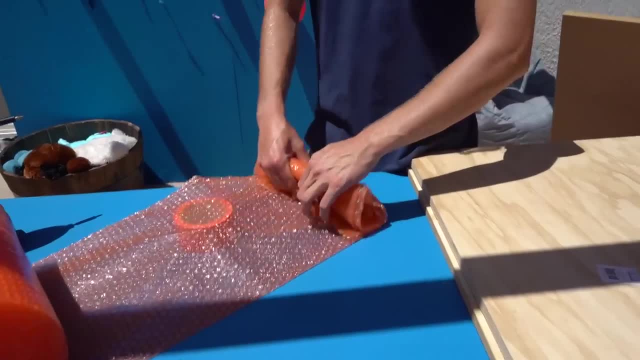 So we're going to just bundle this up, Then we're going to try to stuff it into my box, But we're going to need a lot of this stuff in order to make this work. I don't want Chris' phone to break on accident. 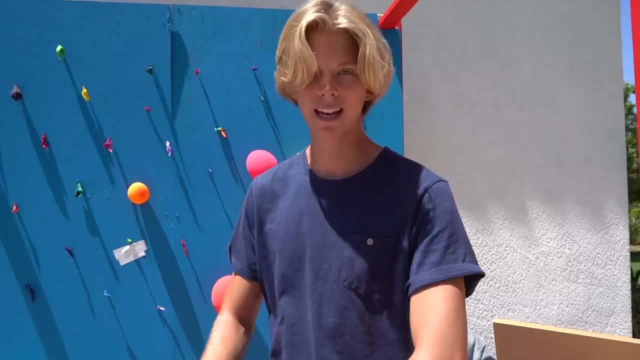 I would hope that they give me the same courtesy. You know what? I think? I've got to wrap this better because my box is actually going to be really small, Because I want to make it small and dense, Because that's like more strong. 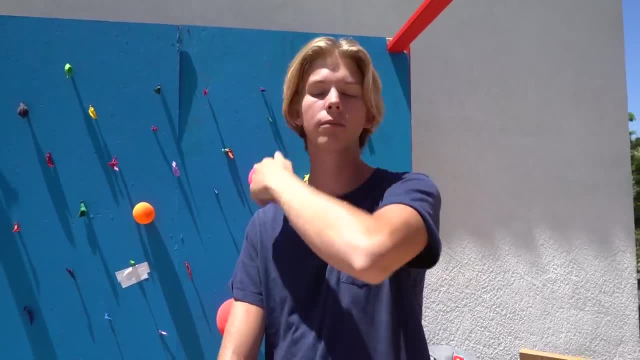 This is going to be difficult. Well, first I'm going to start with making the bottom of my box and see if we can like somehow just barely just get it in there. So we're using these bolts to connect the bottom of my box. 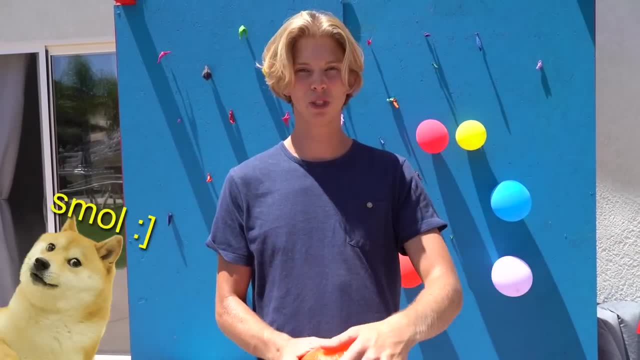 So we're going to use these bolts to connect the bottom of my box. So we're going to use these bolts to connect the bottom of my box Because I want to make it small and dense, Because that's like more strong. This is going to be difficult. 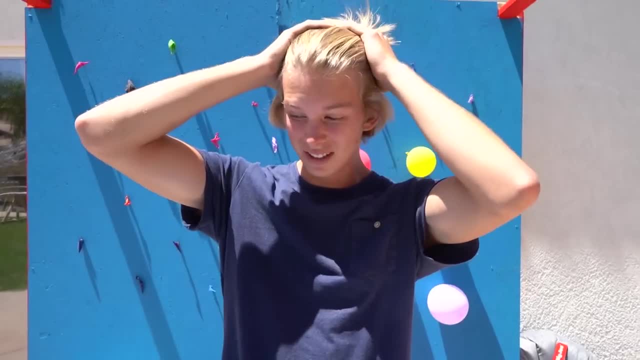 Well, first I'm going to start with making the bottom of my box and see if we can like somehow just barely just get it in there, Because I want to make it small and dense Because that's like more strong. This is going to be difficult. 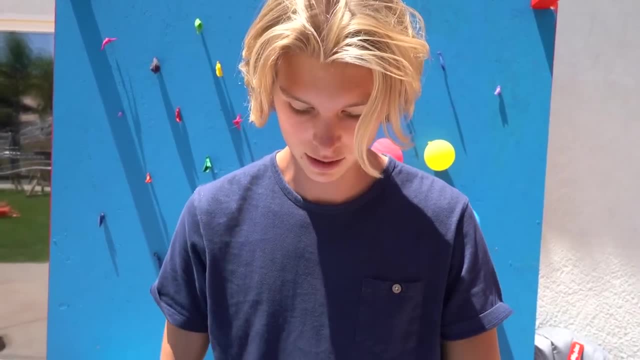 Well, first I'm going to start with making the bottom of my box and see if we can like somehow just barely just get it in there, Because I want to make it small and dense Because that's like more strong. This is going to be difficult. 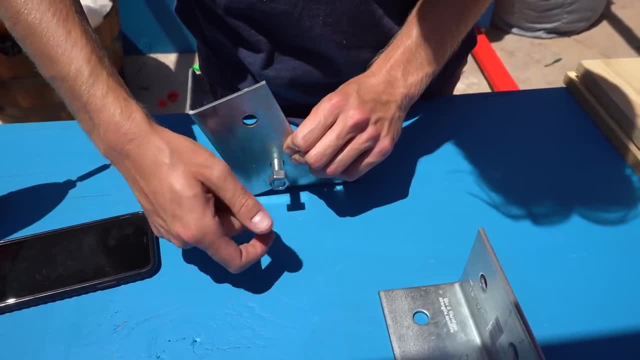 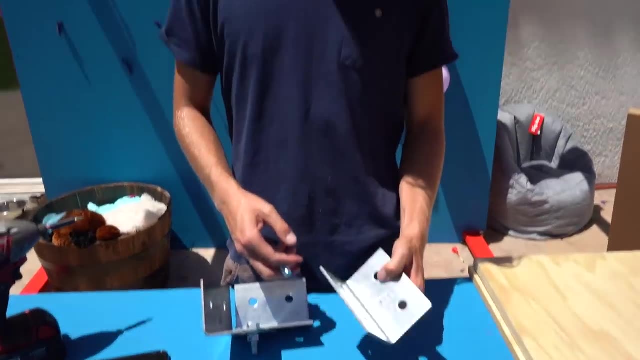 Well, first I'm going to start with making the bottom of my box and see if we can like somehow just barely just get it in there. So we're using these bolts to connect everything, Okay, Okay, so first we first. we got to disconnect these four brackets here. guys, if we can actually successfully do mine, 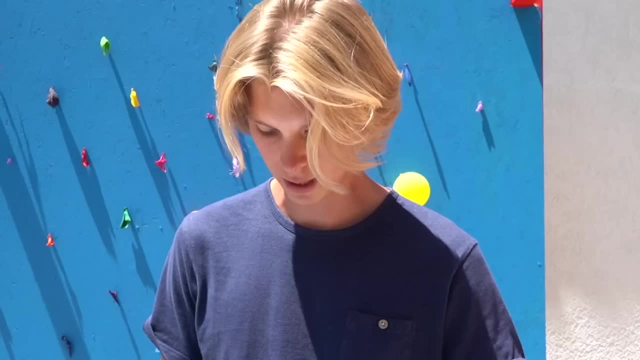 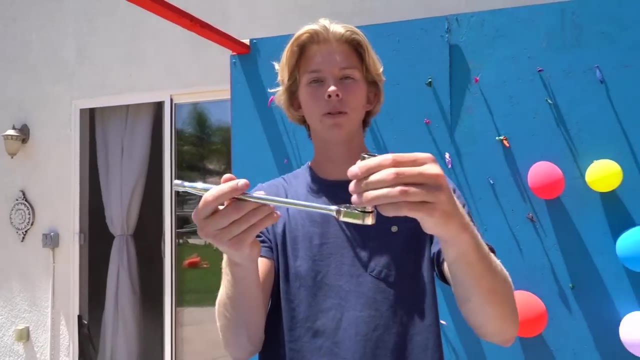 I think it's gonna just blow all the competition out of the water, because this is some thick metal with some thick bolts. Okay, Now I just got to tighten these off really tight, So we have this wrenchy poo- Very fancy. getting all these bolts tight is going to be a squeeze, because once this thing is enclosed, 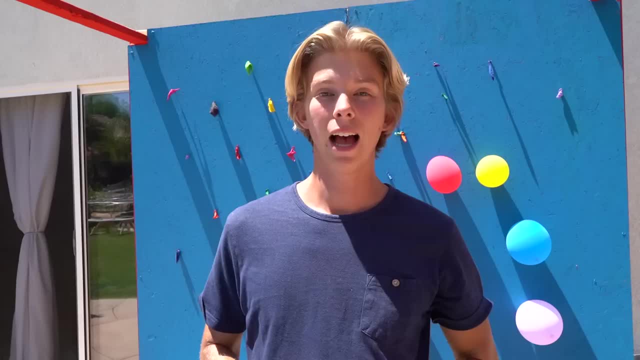 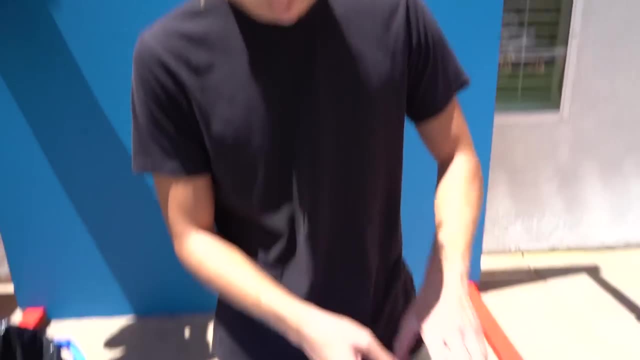 It's going to be hard to tighten everything. I Got a couple more bolts of time and then we can turn any more brackets. Hey Rob, Hey Ryan. So right now I wrapping up Jeff's phone, So I'm making a one foot by one foot by one foot box. 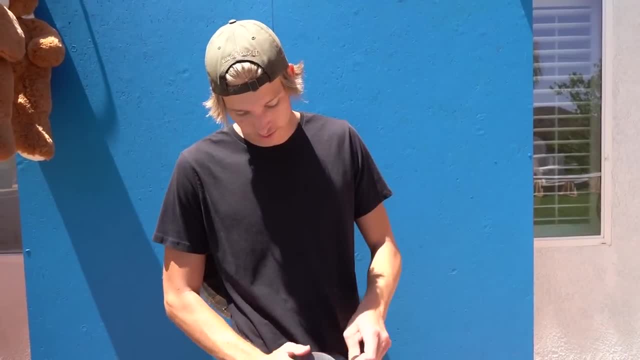 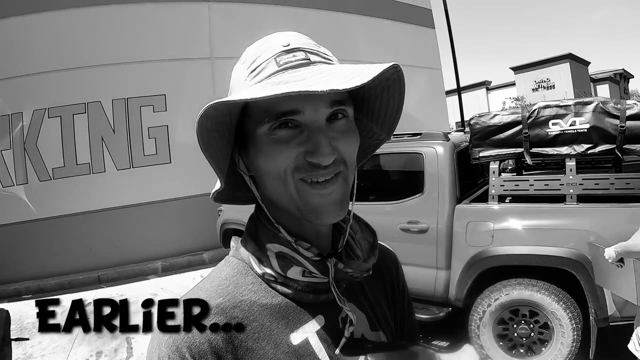 I think this is pretty good. I hope Chris wraps my phone up pretty nicely as well. Ryan, who do you think do where? yes, use question. Who are you you think is gonna win? Yeah, you say again. I remember probably Rob's, Just looks like some c4. 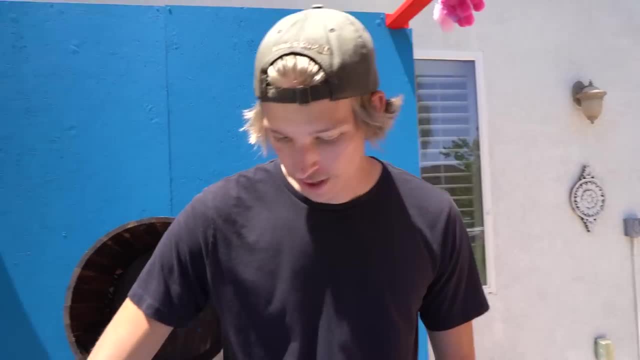 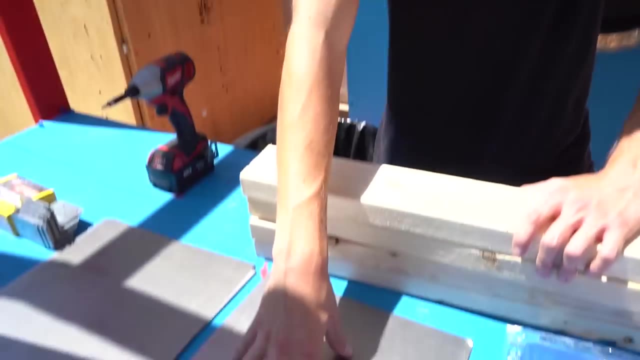 Oh, Anyways, we're gonna head over to the cut station and then work on our structure. after this is done, We're gonna put Chris's phone in and then we have metal to wrap around it. We got these brackets and I can't see a pretty strong box. Oh, 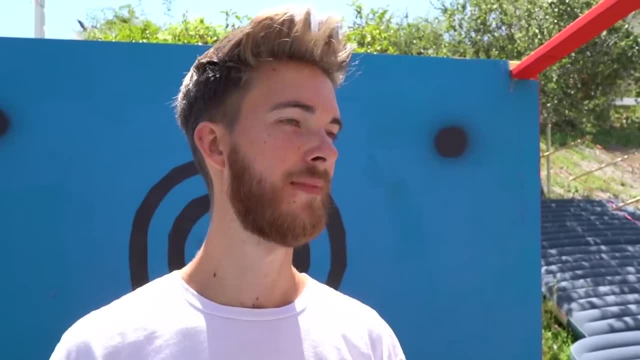 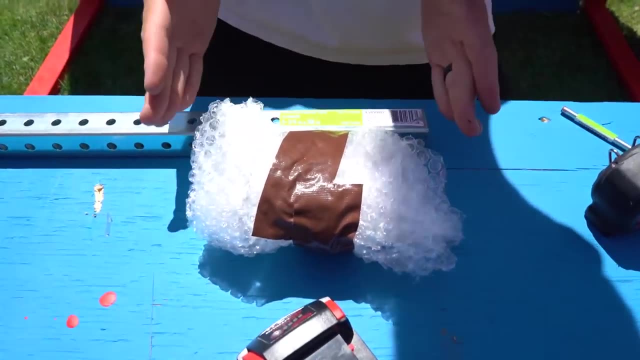 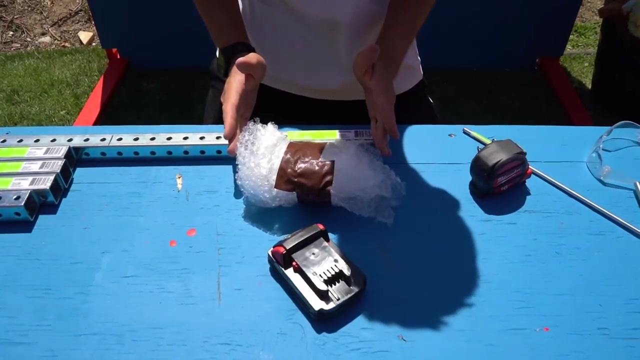 Hiya, hey, Chris. okay, Other people always make noise when I go to talk, So I got Jeffrey's phone right here and if I make my box this big, This is Robert's phone. So if I make my box this big, Then his phone will fit in there. 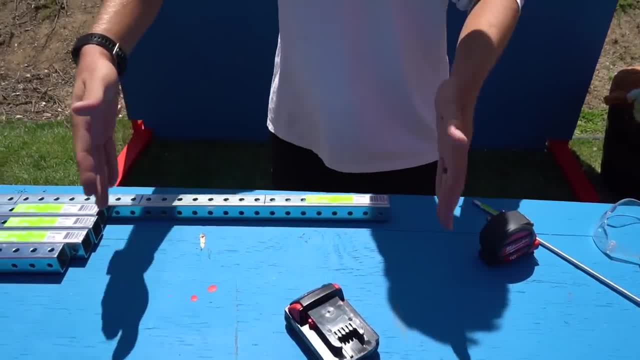 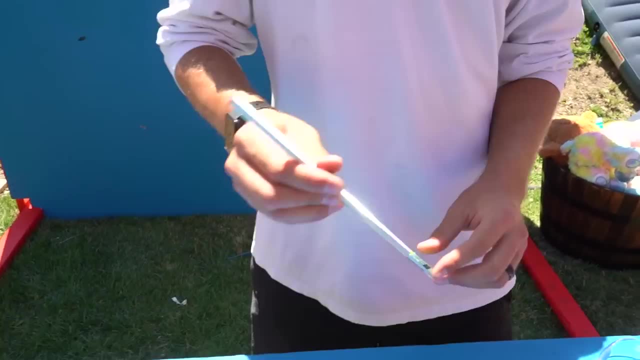 so I'm gonna basically make a wall, like each wall, out of these, and I'll be able to drill holes through everything and put some Nice strong bolts on there. I got these which will go all the way through and really strengthen this box. honestly, I think this box is gonna be pretty dang strong and 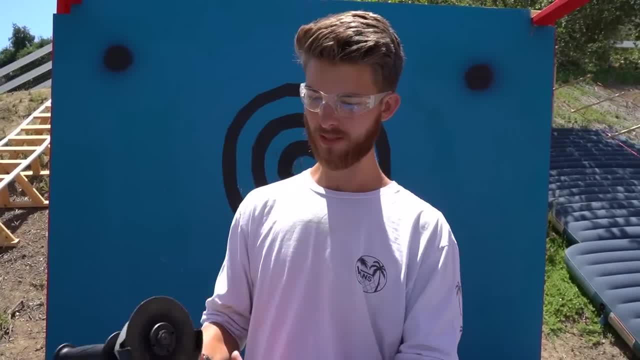 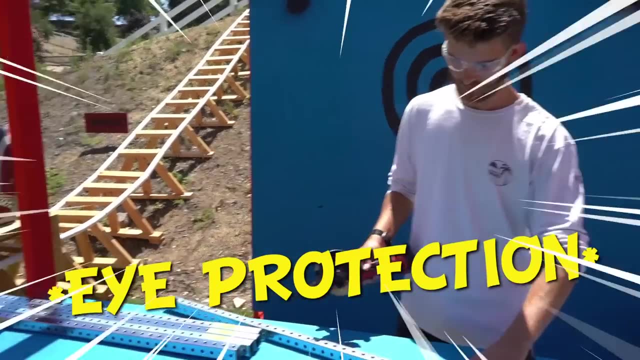 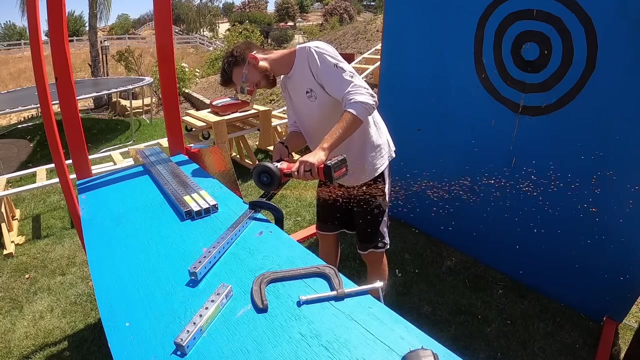 Rob won't be able to break through it with any measly Weapon, so I got to use this thing. It's a little bit dingy, Brian, You might want safety glasses. Here we go. That's why I'm standing all the way over here, one down. 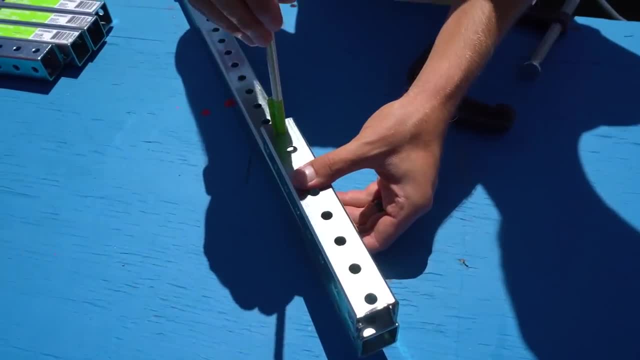 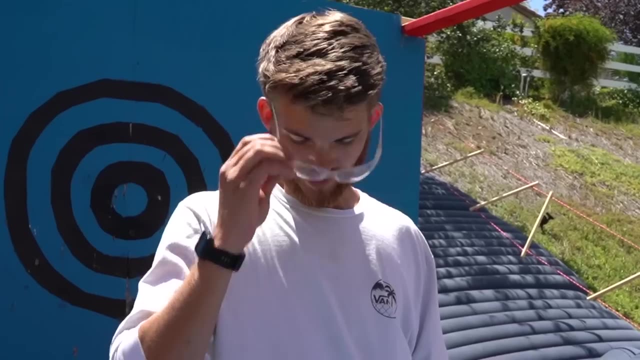 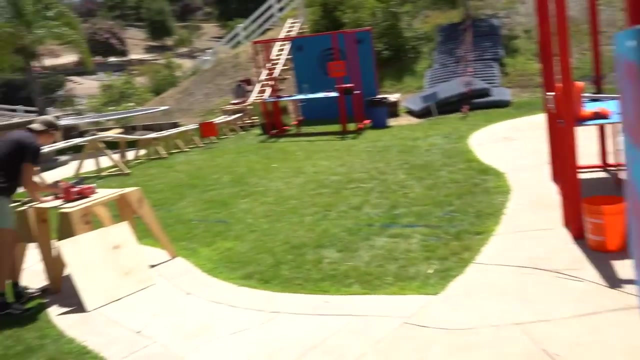 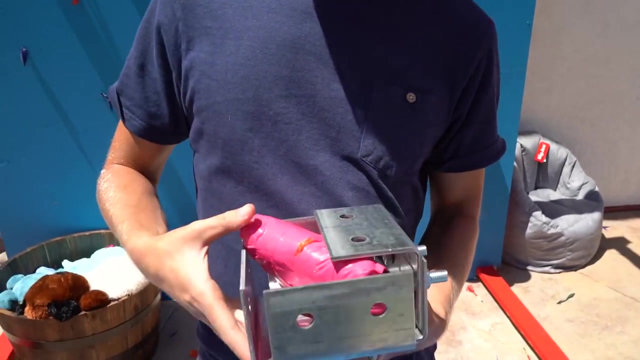 So I'm gonna stack it like this and then these bars are just gonna go through there like that and just kind of like really reinforce this. so that's kind of a Essentially the basic design and we'll see if it works. So, guys, as you can see, Chris's phone is not fitting very well in my box. 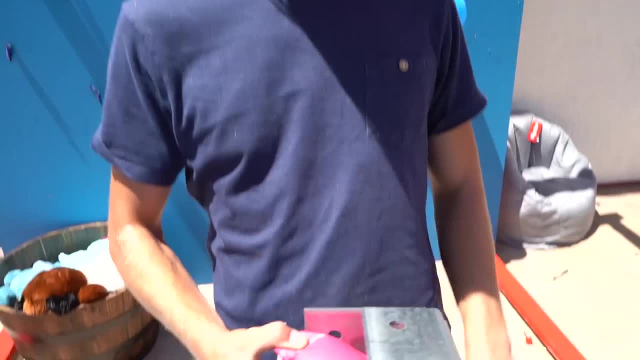 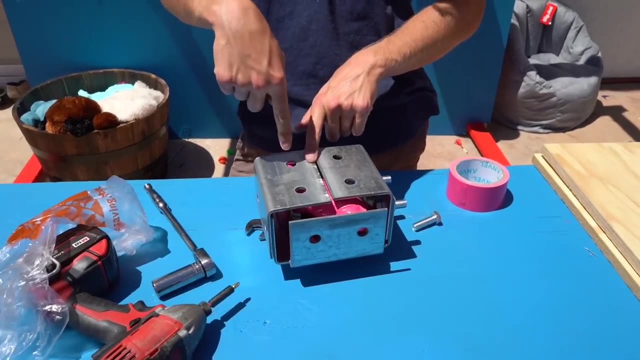 I hope that I can get this thing to be more in here, because this is unfortunate, But I may not be able to use all my brackets that I wanted to. I made this have to be something like this: cuz Like the bolt will go into the phone like that, So no. 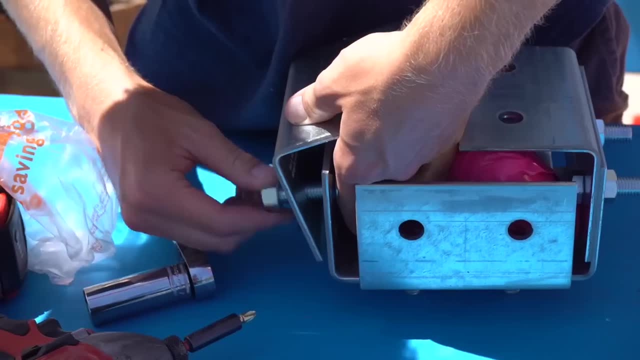 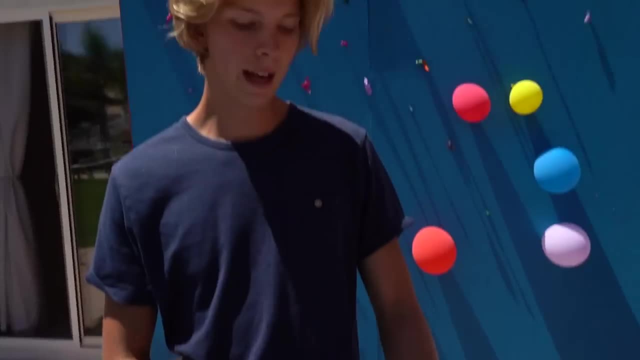 No more crying, only action. So my final idea was to like put this like this, as you guys can see, and I might be able to do it, But I don't know how the heck- I'm gonna really get this on tight. and look at the holes: don't even line up very well. 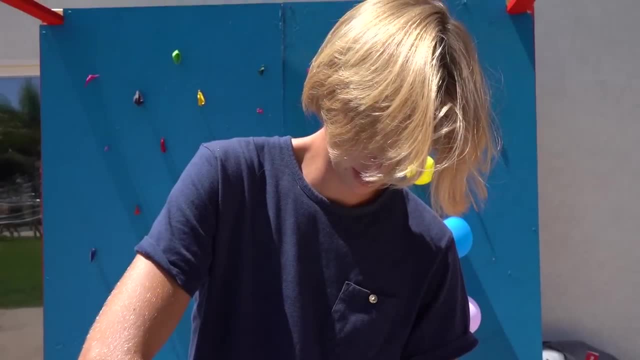 So it's like: what do I do, Ryan? you like what you see right now? Yeah, do you think this is pretty good? Mm-hmm, Yeah, I think I'm gonna be the most successful out of all of them. Yeah, you really think so? 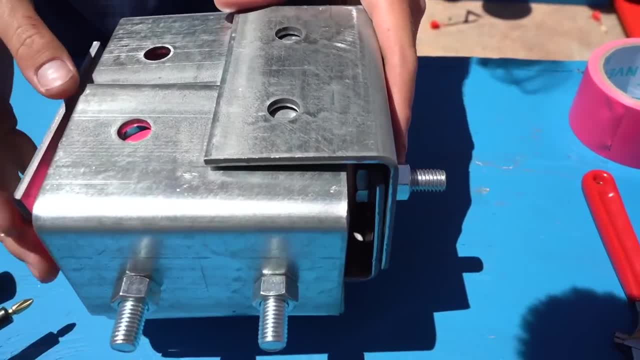 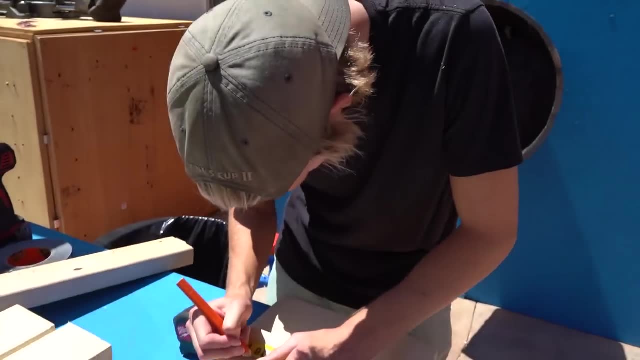 Mm-hmm, Probably Rob's good. I mean, this is thick too Like there's no getting this. if I can get this totally sealed tight, There's no breaking this thing open, dude. Hey Ryan, so I heard um, how do you think Jeff's gonna win? Oh, oh no. 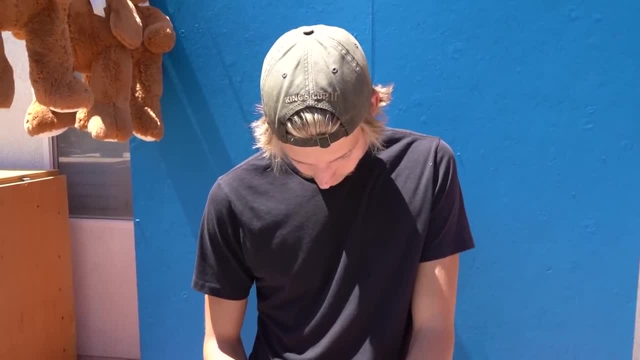 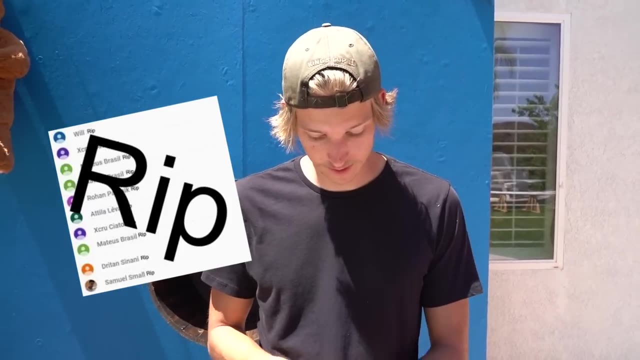 I think maybe all you guys will win and you'll all have to throw away your phone. do that suck, dude? I got a lot of memories on my phone. That's no, bro. Oh well, I can't anymore, Which is a big rip in the chat. if you ask me, you know, if you guys are generous, press after pay respects. 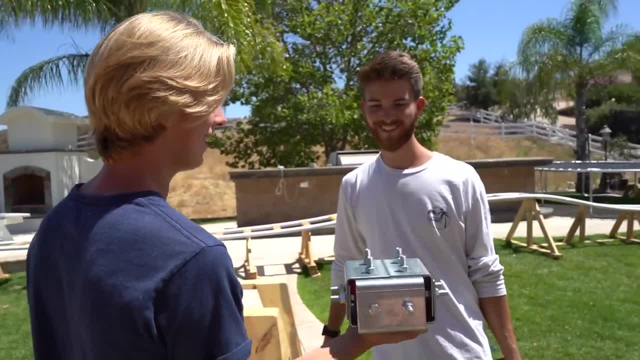 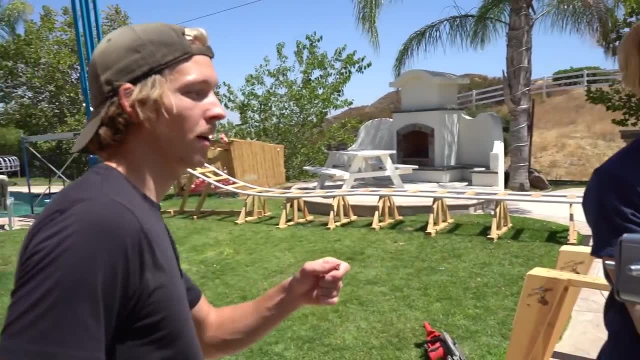 Hey Chris, Check out my box. Check out my box. I just feel that your phone is in this monstrosity. How did you do that, dude? That's thick metal. You're not good at your phone, dude. That's why I wanted the block to land on red. 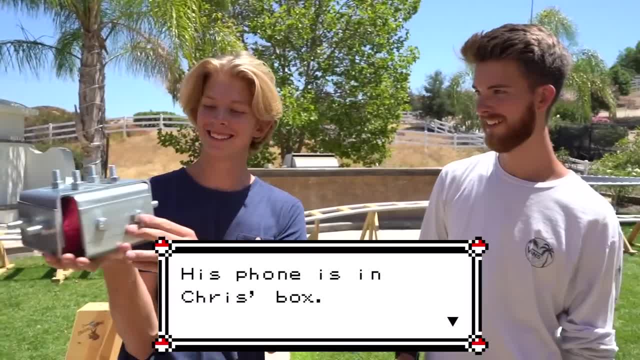 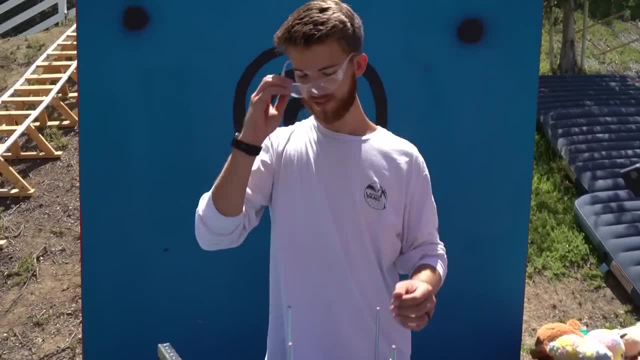 So I wouldn't have to have my phone in this death because look out, look at this, This is steel with steel bolts. This thing is hecka strong. Good luck, dude. You need a new phone tomorrow. So you can see that my cube is starting to form. 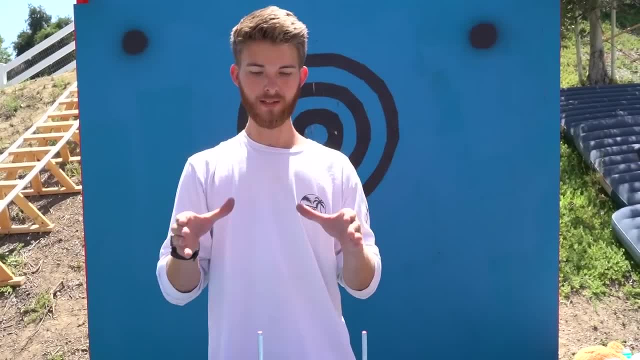 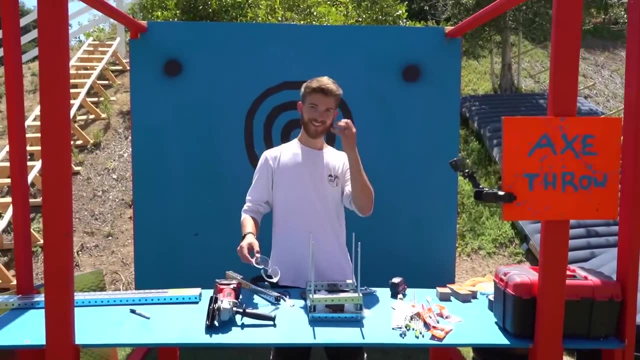 We got these really solid metal bars that are gonna make the structure of the box. I got a lot of cutting to do, so that might be cutting For a while. you look like you're building some kind of like crazy Fighter robot over here. a battle box is gonna fight back. 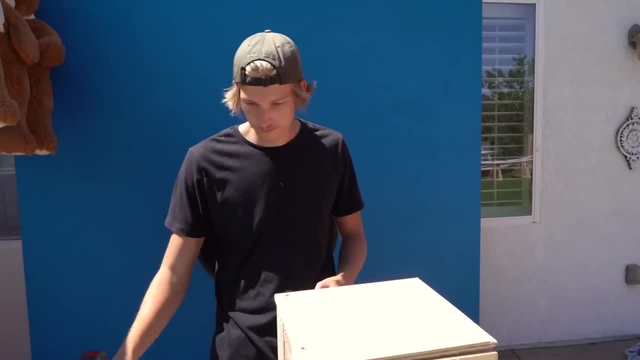 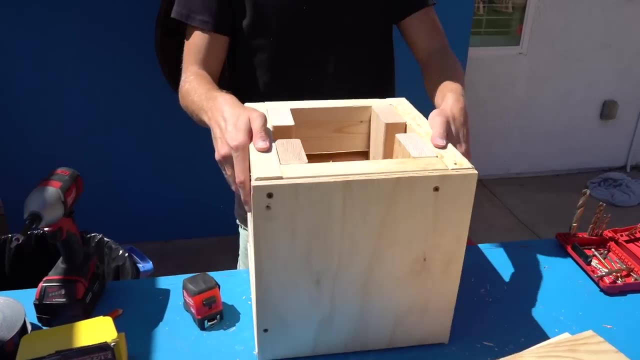 How does it? pretty good, we're finishing the frame of the box and then Show you: well, even this side open, because then that's where Chris's phone is gonna go boom, right in there. Oh, At this point I don't even know. this one I have. 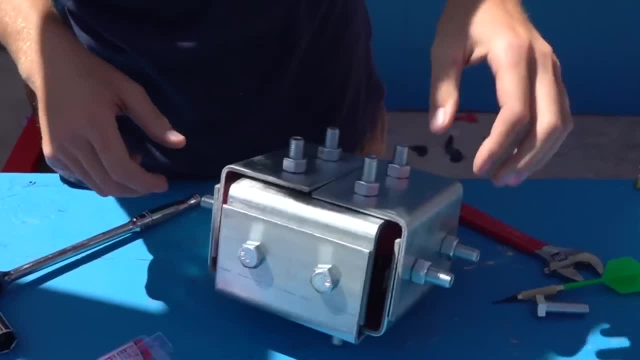 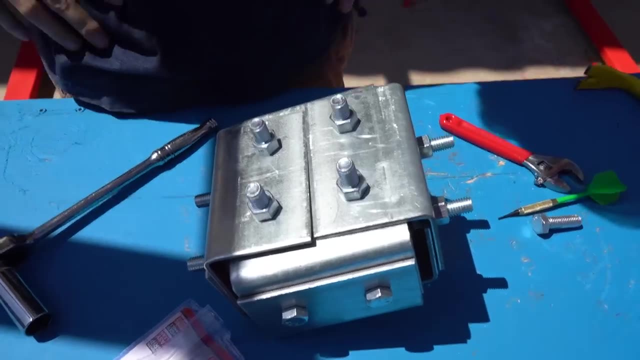 So, hi guys, I've gotten all my bolts on. I'm just tightening them all. it's not gonna be perfectly like like square because, as you can see, like it's kind of crooked. That's just because Chris's phone has been making it difficult for me to get it on straight and like locked in. 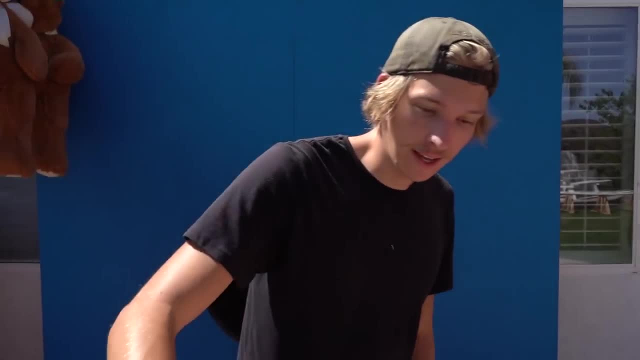 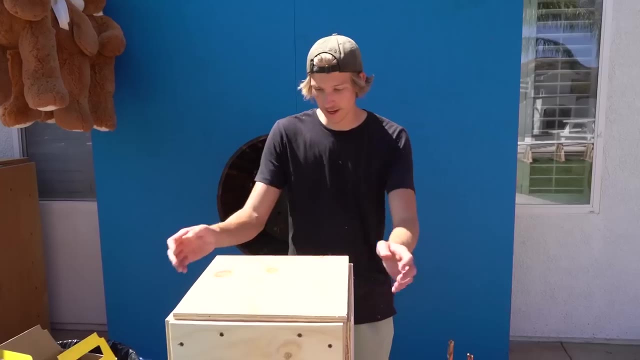 So I don't know, but I still think it's gonna be really strong. So every side, there's plywood on in there now. So now he goes, Jeff's phone never just be seen again, Right, Jeff guys? that is a box. once this is done, We have these metal sheets. 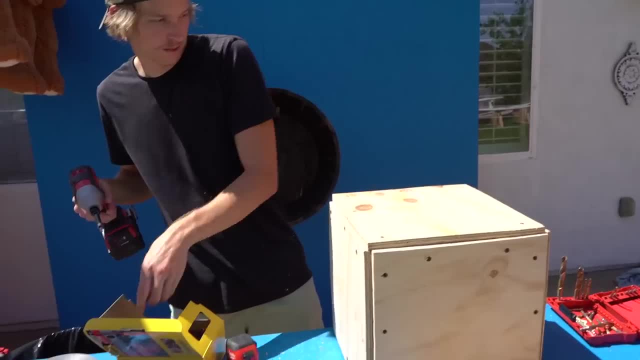 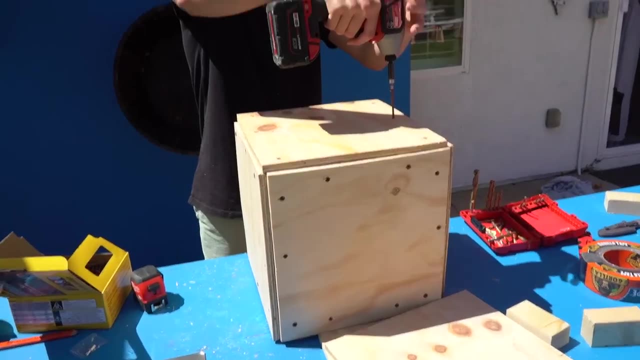 That are gonna be followed by these metal brackets. It's gonna make it super strong. does this remind you of the, the Cuban transformers? Oh, oh, the Shia LaBeouf days? Yeah, yeah, except it's not blue, doesn't glow blue? What do they call the tesseract, or something? 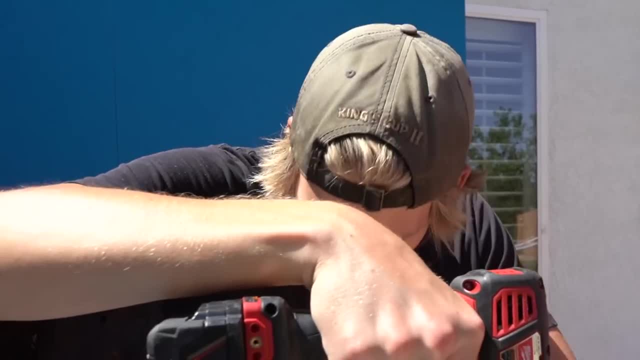 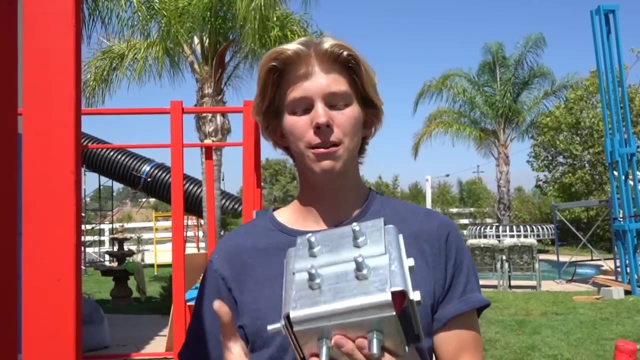 Do we don't? we don't know our transformers very well. We should look it up. Hey, Siri, Guys, we don't have any phones and look anything up. but, guys, I think my cube is complete. all these bolts are on as tight as I could possibly get him. Chris, check out your box. 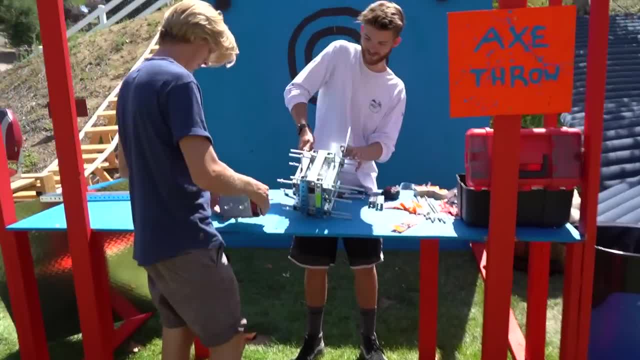 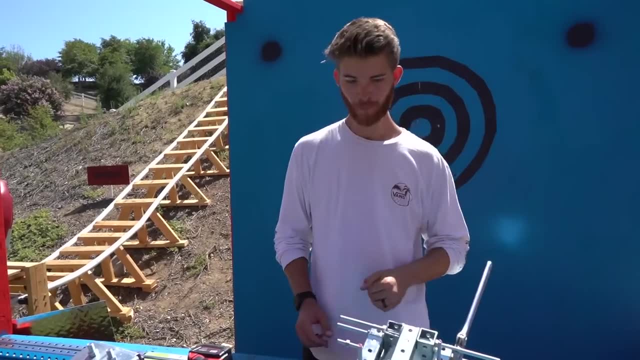 Dude, I like how you say: come check this out, But you come here. That's true, Take that thing out. That's just pick it up. No solid, That is no way. This is cool. This looks like really interesting. I'm just looking at it. Well, I'm done with my box. 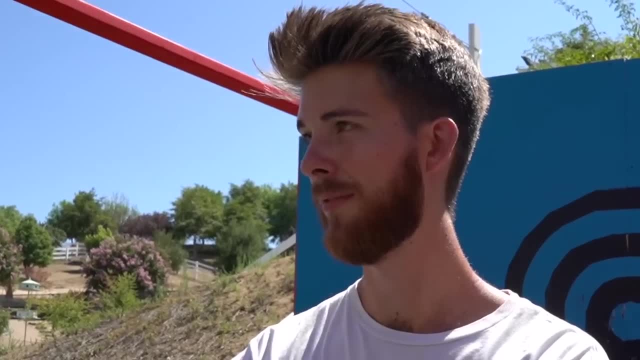 Shut up? No, you don't. You think I'm bluffing? Call me on my bluff. Then what's the weakness? I'm telling you, I'm just gonna wait and see you cry when I open it. I ain't worried. So you almost done with your box, Chris. 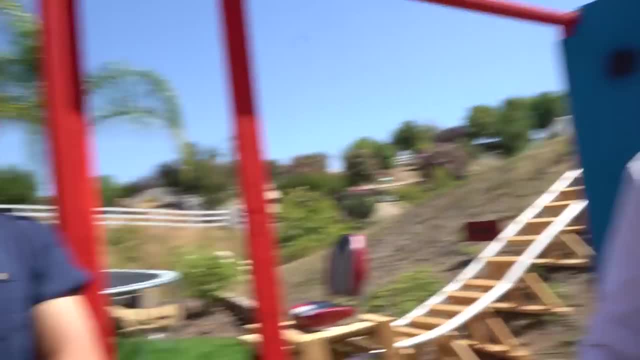 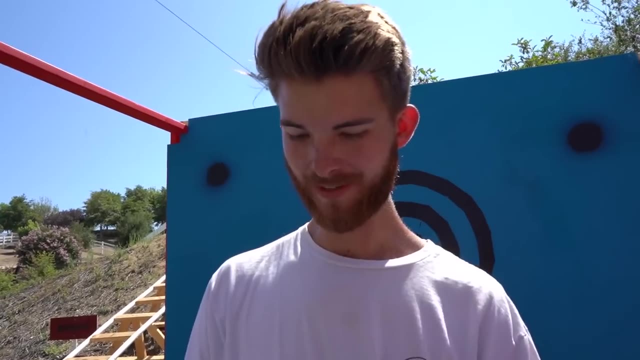 No, I could add like 20 layers of metal, because I see, when I see many weaknesses with yours, Oh yeah, Did you? I don't even done yet, dude, I do, though. You're just trying to make me feel bad, huh, Nope. 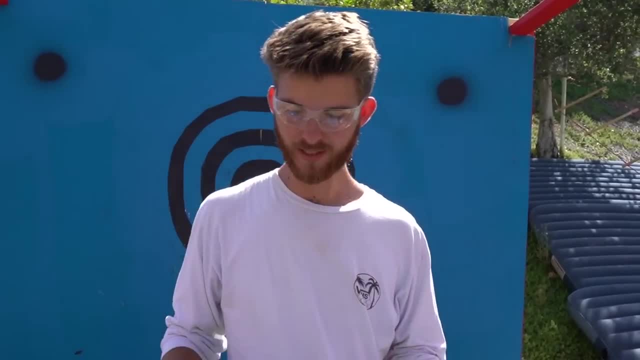 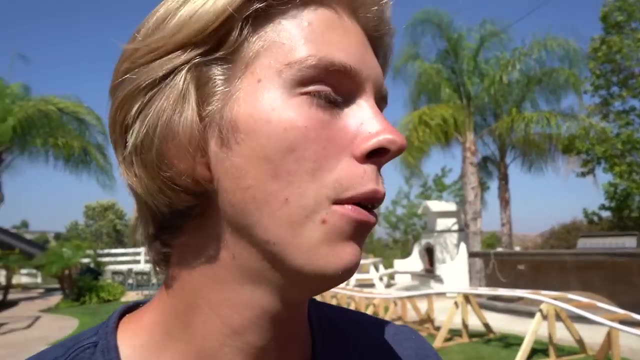 Anyways, I decided I'm not gonna put the metal sheet on top. I'm just gonna try and make it so that Robert can't squeeze the phone through. guys. It's been like an hour since I finished. Robin, Chris are still working on their boxes. I may or not, may not have drilled through Robert's phone. 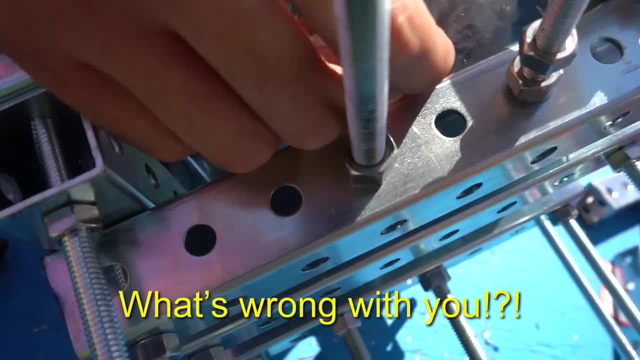 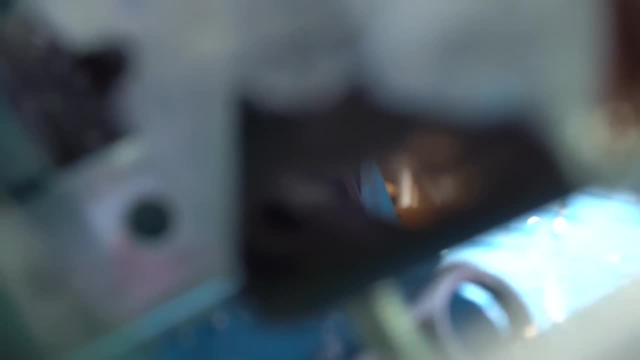 Oh, Did you do it? Oh, I think it's fine. I think it just went through the tape. Chris, you have to be more careful. Dude, that was actually really close. Let's go check on Robert's box. Roberto, Dude, your box actually looks cool. 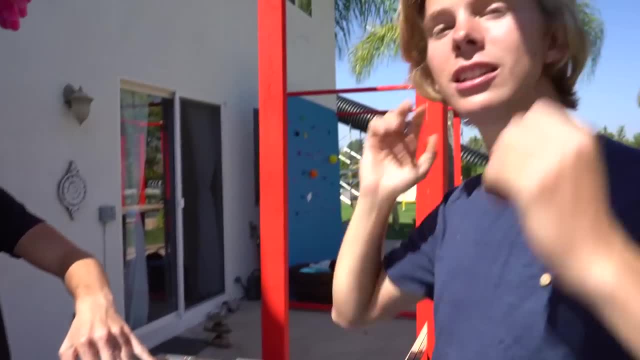 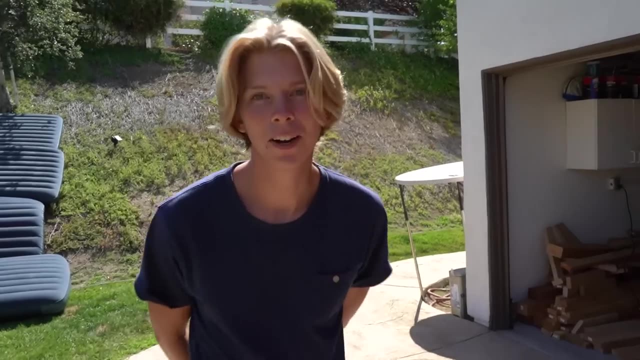 You've got these metal plates and these metal brackets and it actually looks pretty neat. I still think my box is the strongest. Alright, let's mess with Chris While he's moving. Follow me, follow me. Where are the wiffle balls? I don't know. 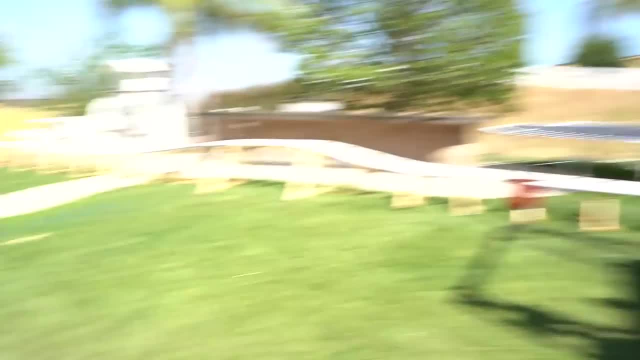 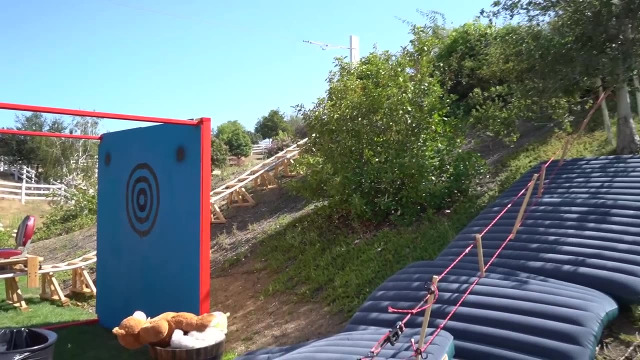 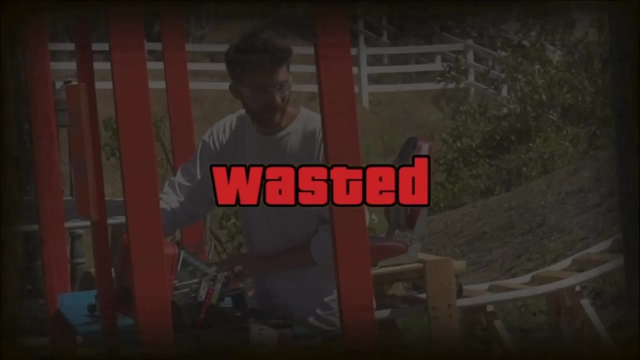 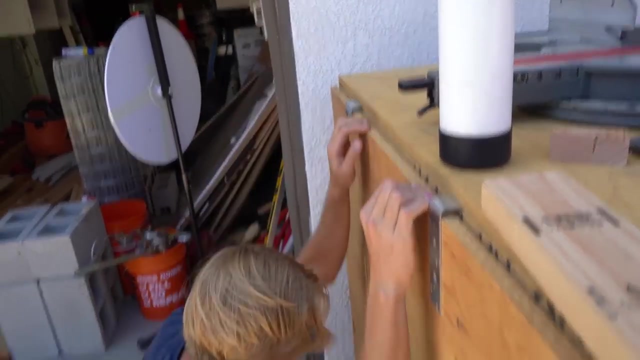 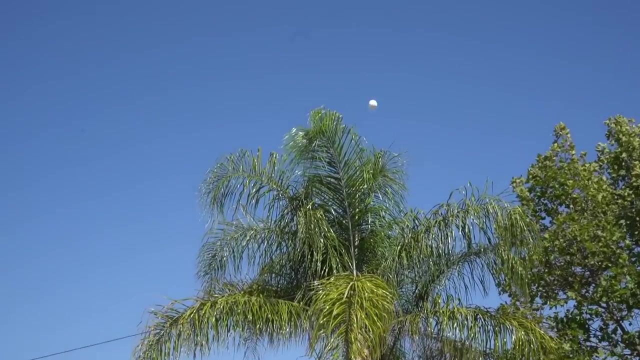 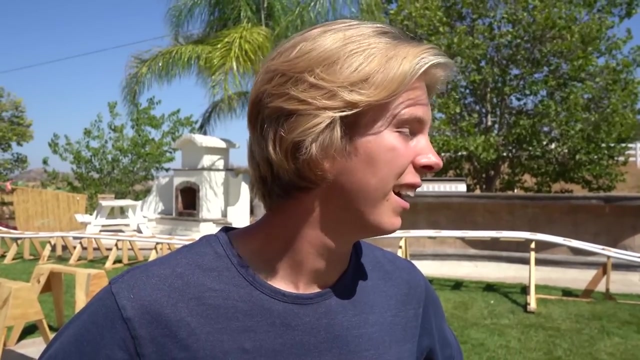 Chris, where's the GoPro Right here? What are you up to Nothing? Oh Oh, Did you hit it, Boing? I don't know how to do it myself, All because you don't have your phone. You're right, This is sad. This is sad. 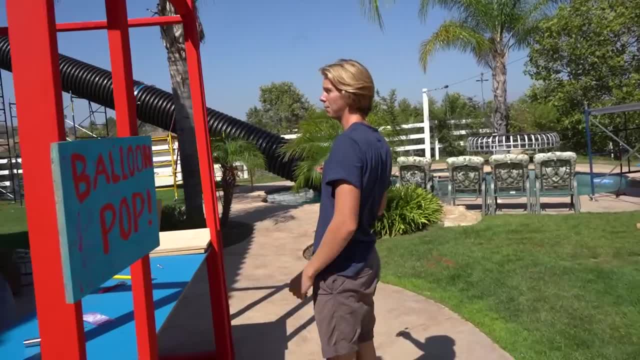 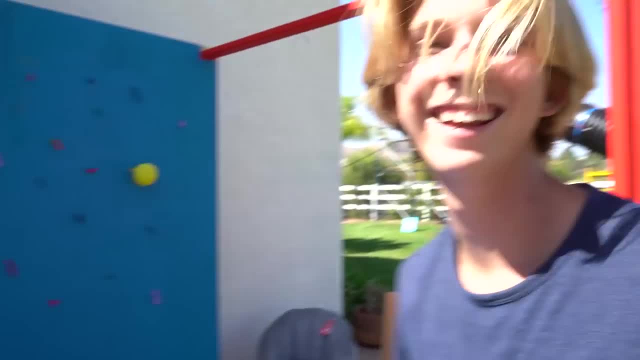 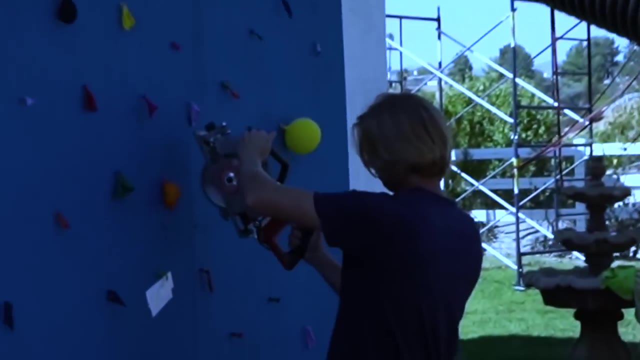 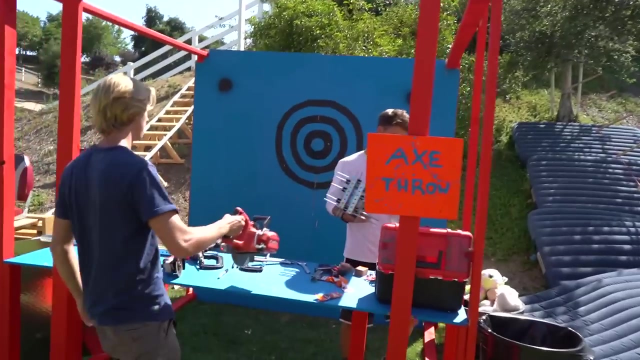 I can live without it. I don't need my phone. I'm going to pop these tiny balloons. I can't hit it. one Still missed. Well, is your box finished? Yeah, my box is finished. Dang, So my name for this one is Battle Box. 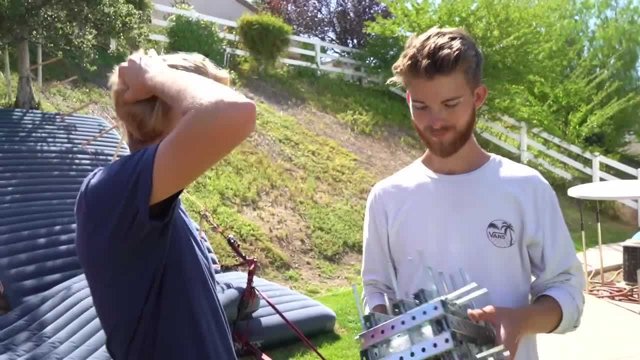 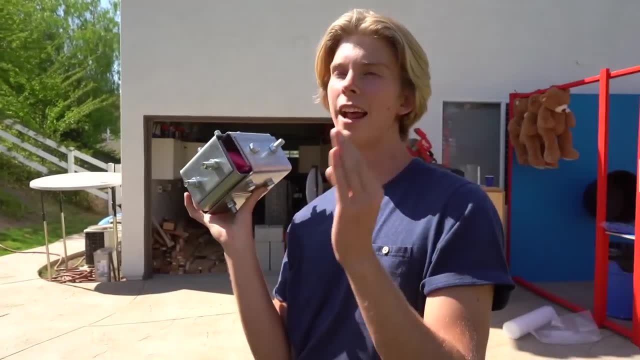 Because it looks like a battle robot. Come look at the box. your phone is in, bro. I gotta figure out my box. I'm calling this Eggshell Why? Because it'll break easily. No, it's an ironic, satirical name, because it ain't going to break like an egg shell. 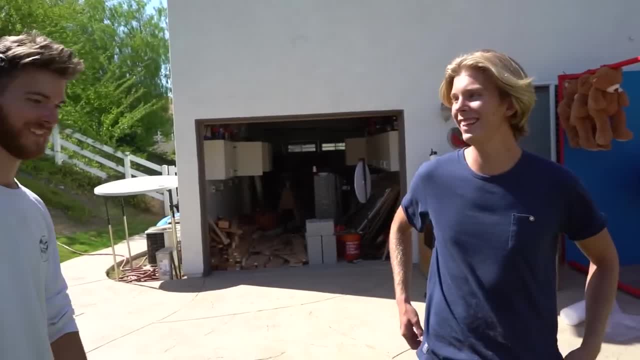 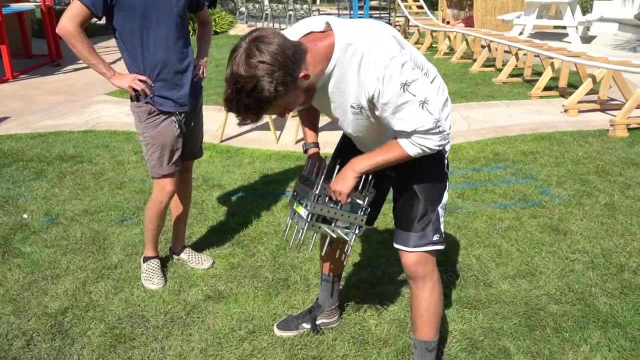 Here it sounds like a janky aluminum can. Good luck, Chris. Hey, my phone's in there. Oh, it's not even in bubble wrap anymore. Are you serious? Because the drill took the bubble wrap off, Dude? look at what Chris Dude, he can just pull his phone out. 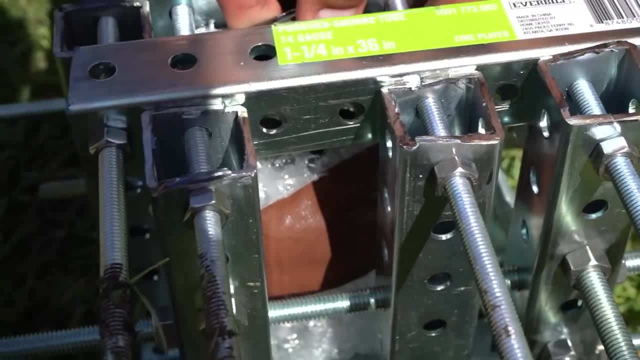 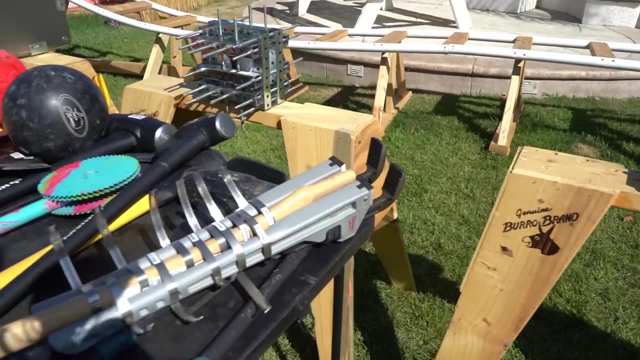 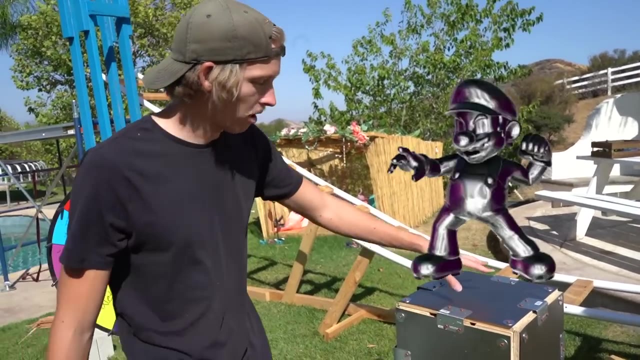 No, You're done. go It barely doesn't come out. Well, you're lucky, Just shove that in there. Subtitles by the Amaraorg community. So it's time to name my box. I'm going to name it the Metal Mario Block. Oh, okay. 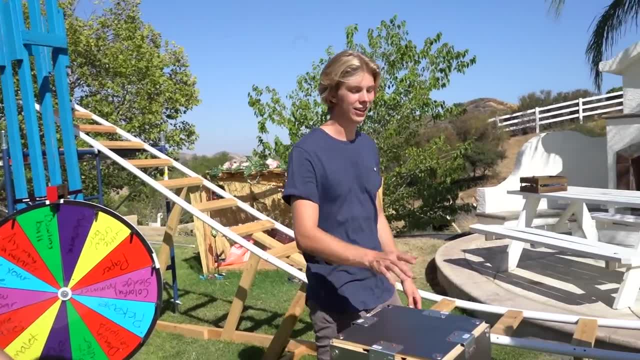 I like it. It looks like a Metal Mario Block. Aesthetically, I like yours the most. I think mine looks the ugliest, to be honest. Yeah, Yeah, you got all these doohickeys just sticking out, But I mean, this part's cool. 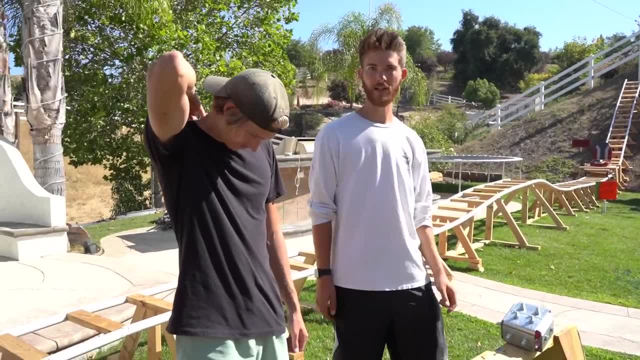 This part's generally pretty cool. I mean, one thing for sure is: you wouldn't want that thrown at your face. So I'm breaking out of this box. Honestly, first thoughts, I think I'm going to be able to get out Robert Robert's breaking out of this box, Rob. 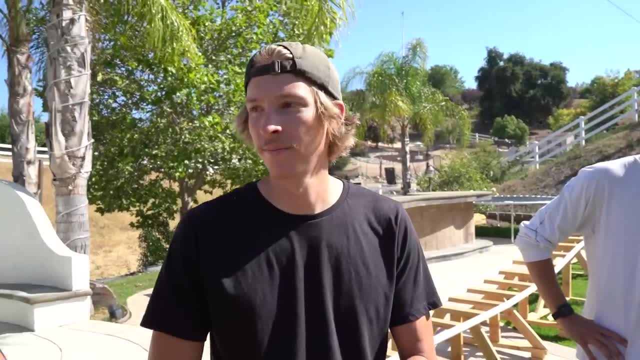 Do you think you're getting your phone out of this thing With the right tool? yes, And Chris, I think you're going to break out of my block of steel- Dude, I don't even know, That's my name for it- block of steel. 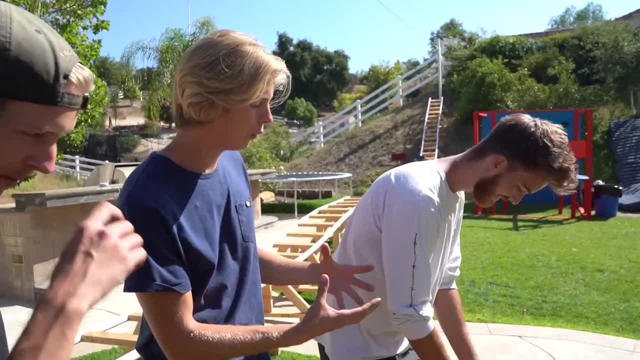 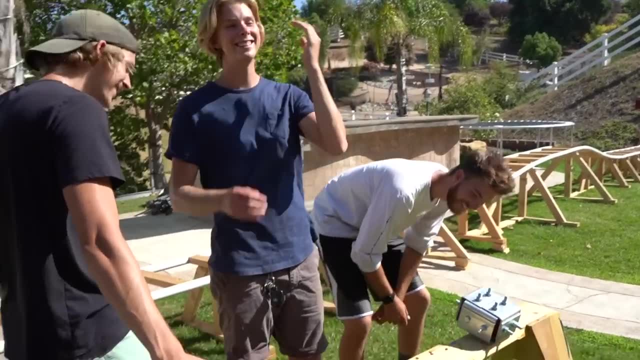 I don't even know, dude. One funny thing about mine, Chris, is it's so confined And the bolts are like pressing up against it. If you smash in the wrong way it's going to break your phone. Oh my gosh, dude, It's so tightly in there that like if you jam it in. 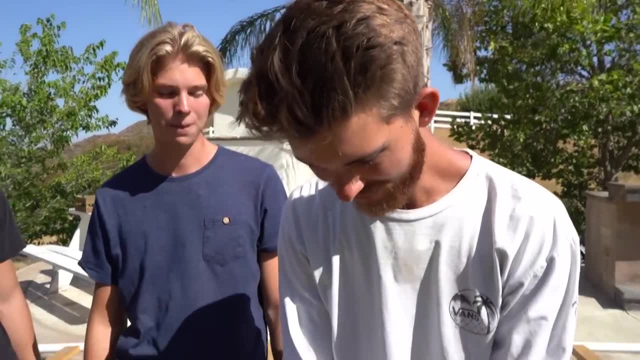 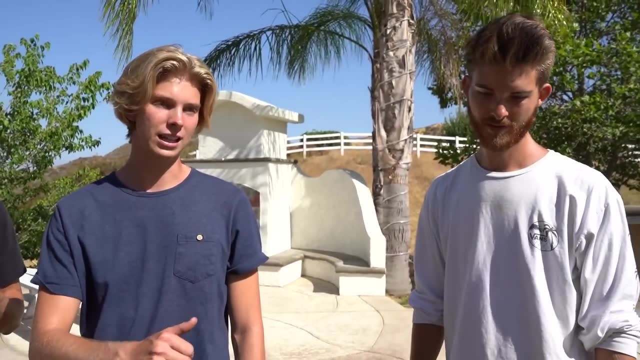 It's going to like cause the bolt to get jabbed into the phone. I think I need to go like for the bolt itself. If I get an axe and I hit it right here, maybe, Yeah, and you have guess what? Four, five, six, seven, eight, nine, ten, eleven, twelve. 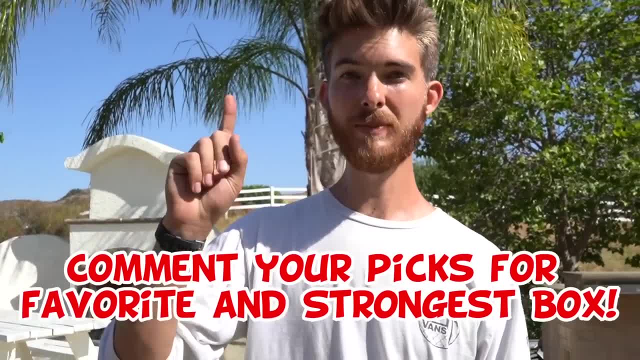 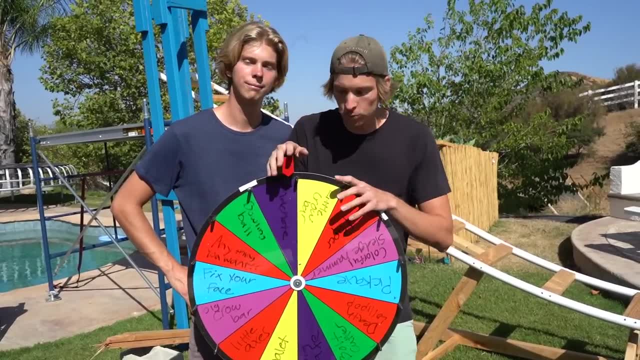 Sixteen bolts together. I'm going to get through. So comment down below two things: Which box is your favorite and which box do you think is the strongest? We're going to be using the wheel to determine what weapon we use, So every three minutes we get to spin again. 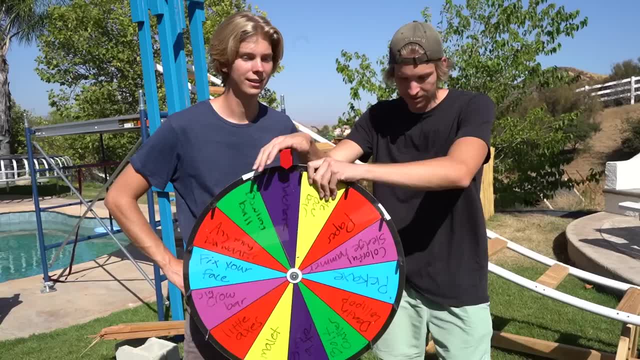 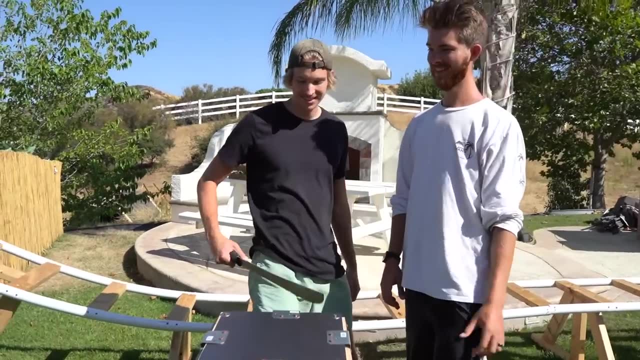 Right, Jeff, Right, Should I spin first? All right, spin first. Let's see what Robert gets. My first weapon is A machete. Here you go, Rob, I'm going to spin for my weapon. Boom, Let's see what I get: Death Lollipop. 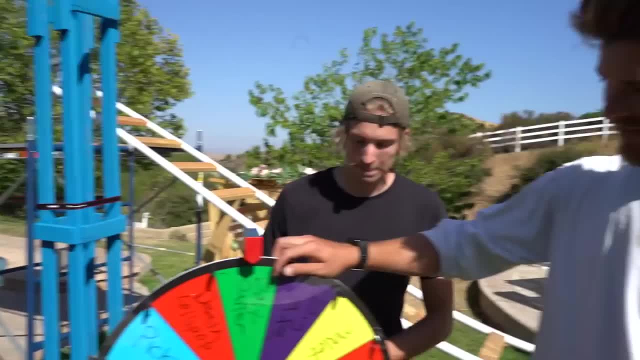 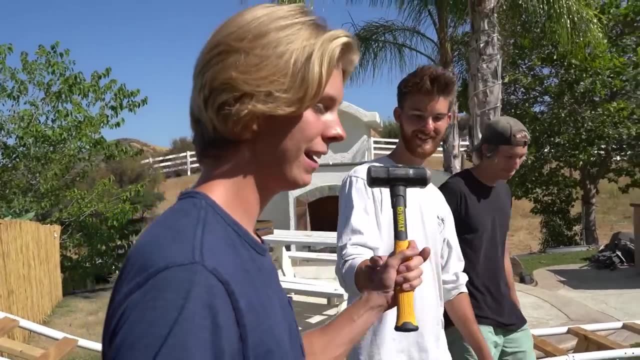 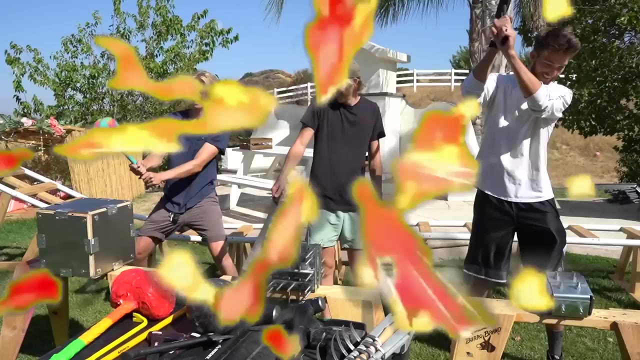 That's the weapon that you made, Dude. I hate that weapon. Okay, my turn, Mallet. Chris, this is your weapon. Not bad, not bad. This is my weapon. It's time to begin destruction. Three, two, one go. Oh no, The box, no. 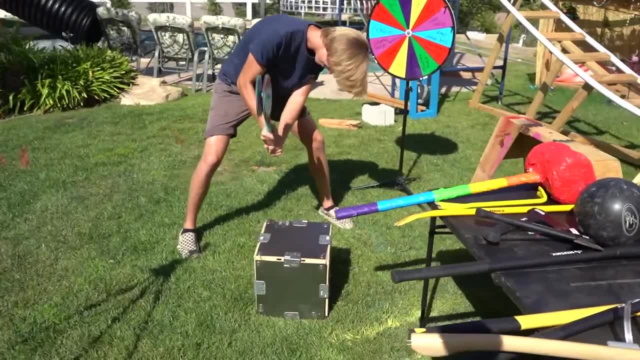 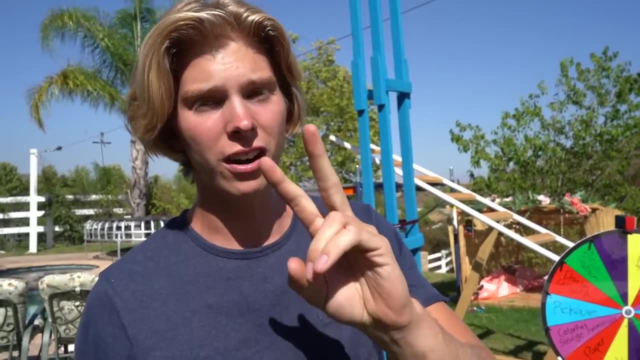 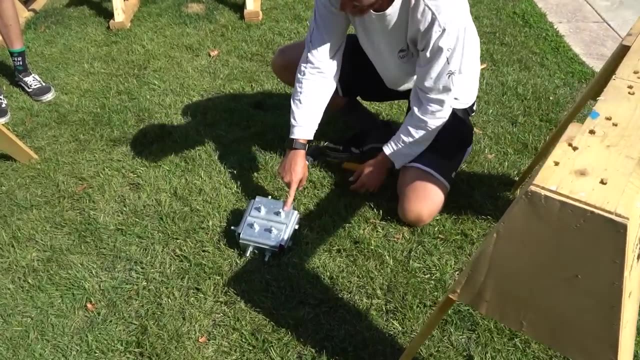 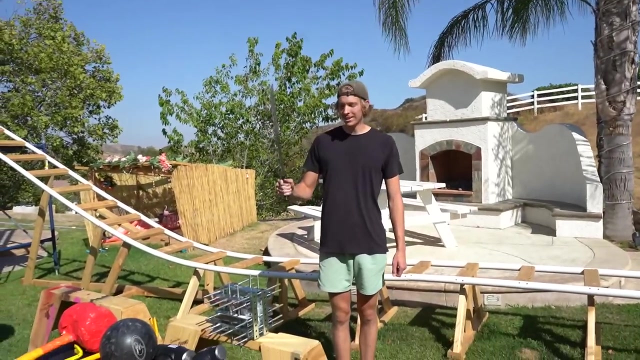 This is not good, Guys. by the way, You get a point if you can get the phone out. You get another point for whoever breaks out the quickest Dude. look at these, I'm bending them. I'm bending these giant screws. Are we blacksmiths yet? 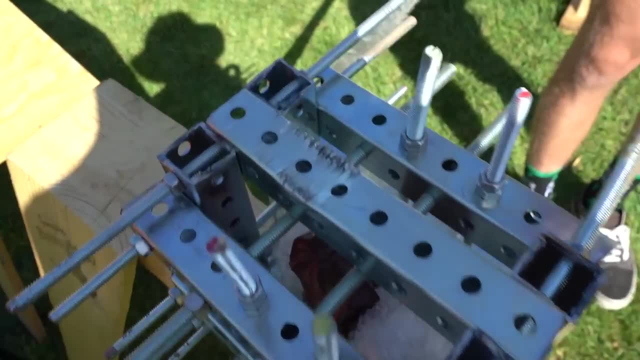 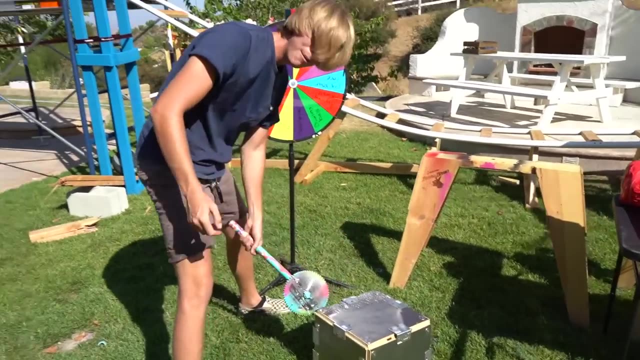 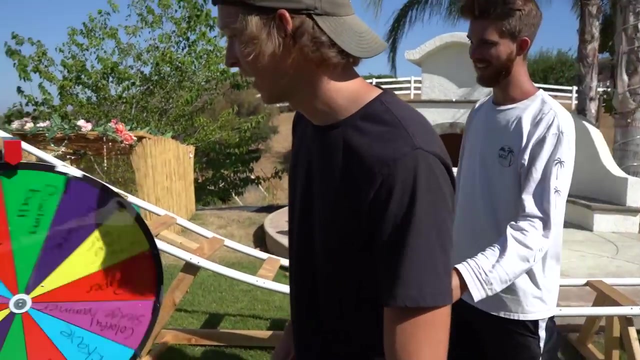 Look at this. It's working, It's somewhat working. Keep going. I'm damaging the metal a lot, Alright, stop, Stop, stop, stop, What Stop? Oh Dude, this is tiring already. My next weapon, Anything you want What? Alright, my turn. I'm tired. 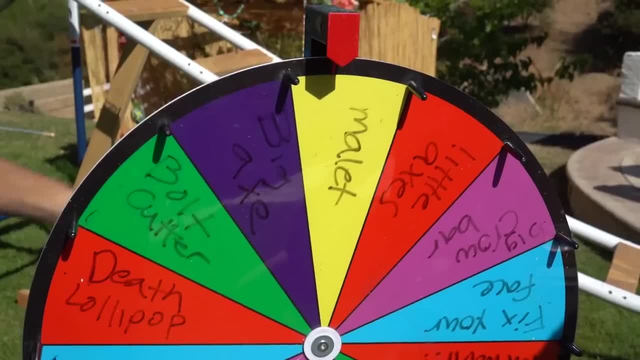 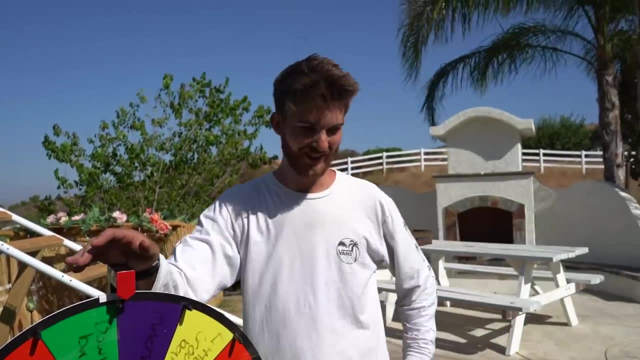 Me too. What do I get? This is so tiring. Oh, I get the mallet. No, Mallet Dude. I was making good work with that, Chris, you got to give the mallet up. Bowling ball, Bowling ball. Oh shoot Guys. look at all this damage I'm doing. 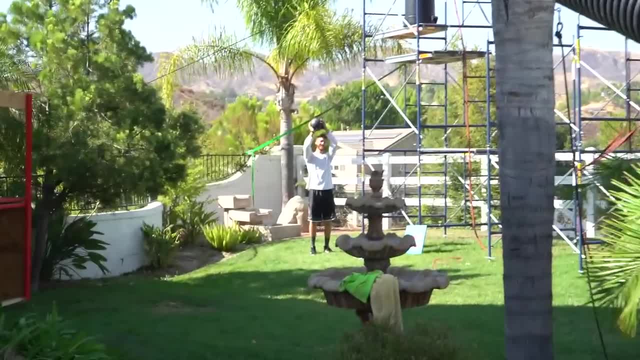 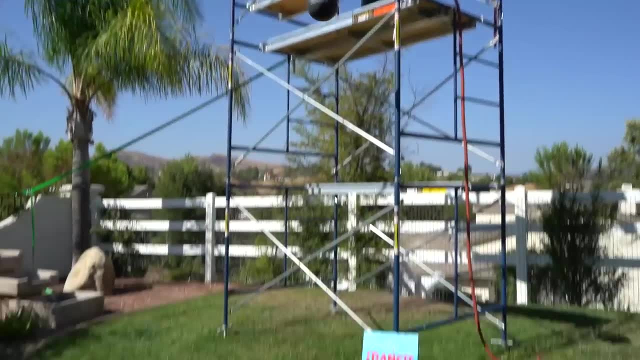 Where did Chris go? What are you doing? Oh, watch out, Follow me. Chris is taking the bowling ball up the scaffold. That's it, I'm going to chuck it. That did not sound good. I don't think it did much. Look at the caveman. 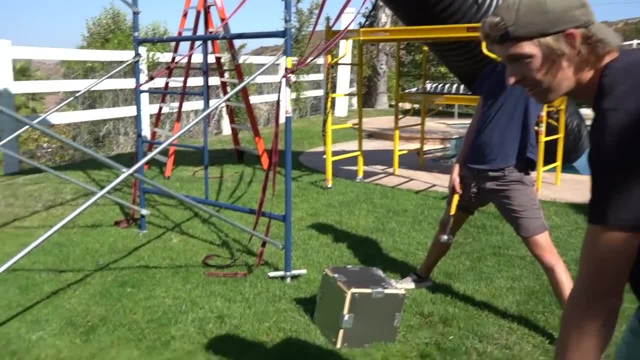 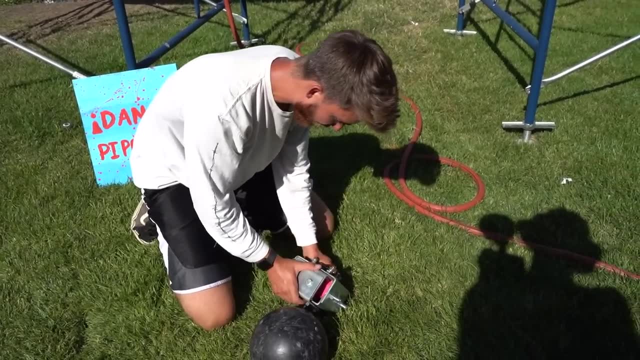 Dude, this box is so strong. I told you: Oh shoot, Dude, the screw is going straight into my phone. What if my phone is ruined already? Okay, I just got to break the screws off, Because if I try and hit the metal in, It's going to ruin my phone for sure. 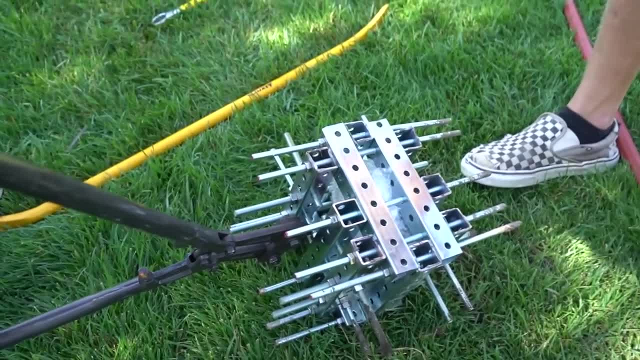 If it hasn't already. Robert's breaking the screws with the bowl cutter. You better be quick, Rob, Because the time is running out. I'm going to break it right at the nut, Rob. I think you're going to get out first. That's pretty OP. 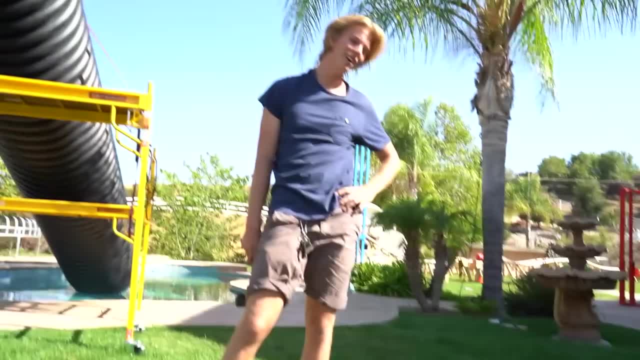 All right, stop, Time's up, Guys. we got to go roll again. We got to roll again, Okay, well, now we got to re-spin. Okay, spin, Chris, I spin first. Spin, spin, spin, spin. Oh yes, Fix your face. 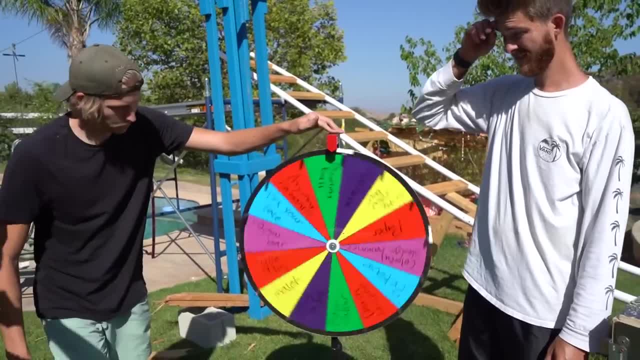 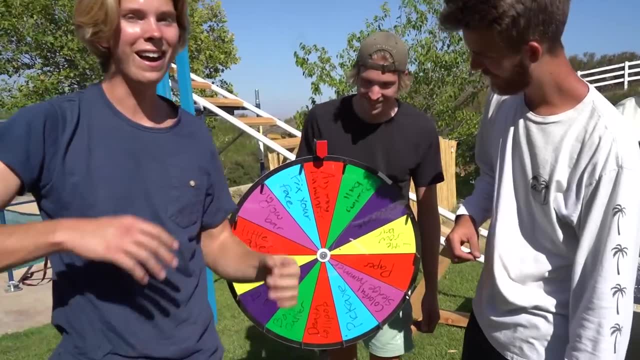 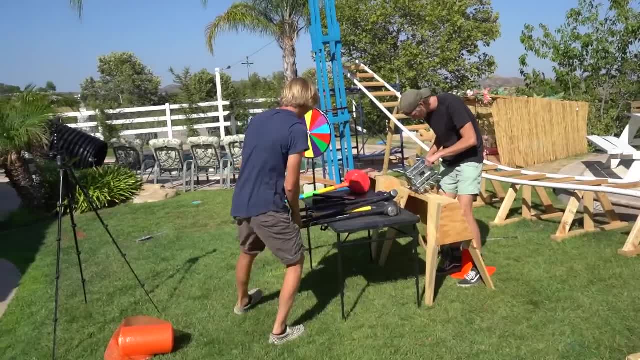 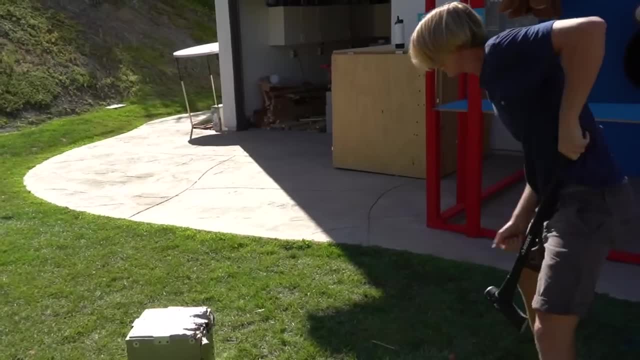 Oh, A little crowbar, A little crowbar. Oh, It's over there. I'm going to take this ax. I think this is going to do some damage. Oh yeah, This is doing a ton of damage. All right guys, What? How did you do that? 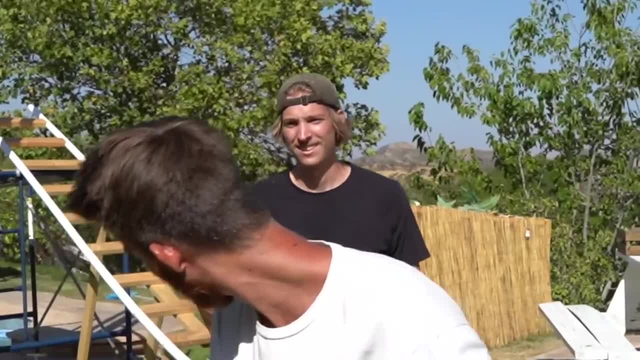 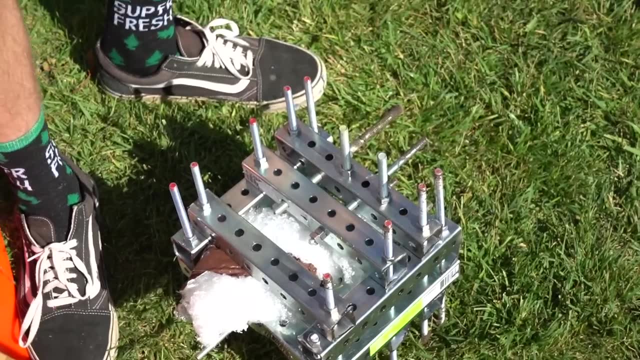 You got your phone. Look, look, look Easy. I tucked the bolt cutters to your weak little screw bolt thingies. My phone was already parked, It was partially out, So I just grabbed it Through the bubble wrap. Rob, you get two points Shoot Because you got your phone and you were first. 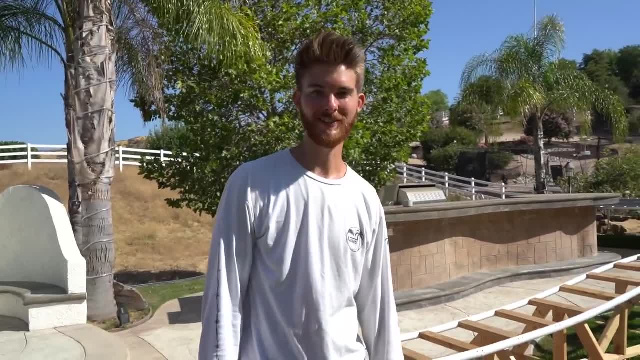 Dude, that feels good. I'm going to go over and see how Jeff does, Because this is the box I built, So that means that my box is the weakest. Rob, is your phone messed up? So it was already cracked, But it cracked a little more here. 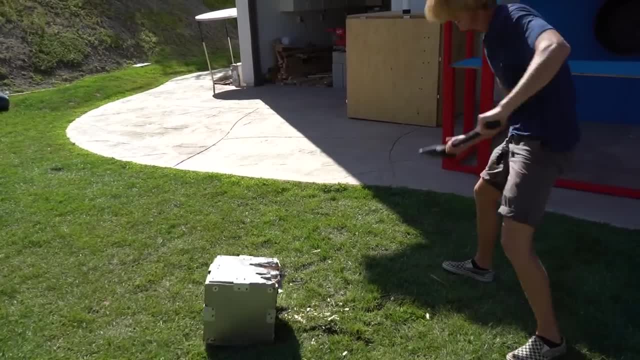 My phone's been beat up. I feel like I'm almost through. You feel like a lumberjack. Yeah, I got to keep hitting that one crack. I'm so tired though. Well, time's up Really. Yeah, Jeff, you seem to be out of breath here. 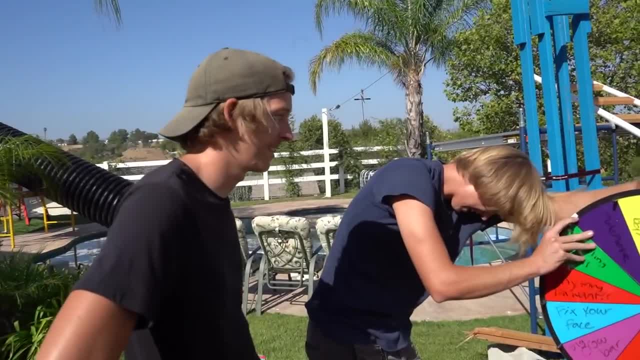 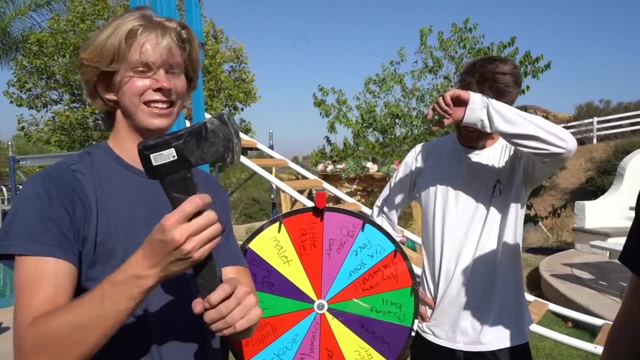 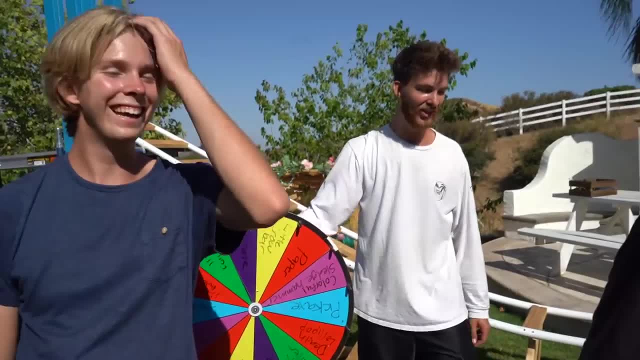 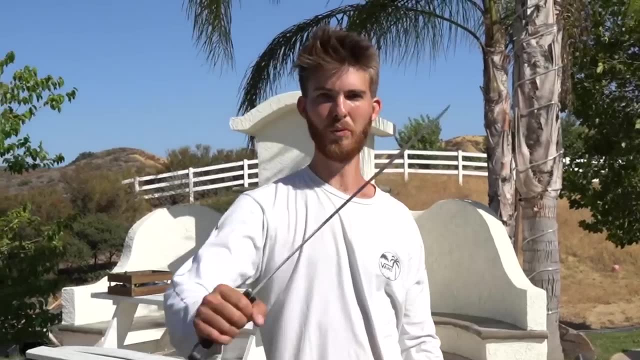 This is perfect Because I can hit hard And also be accurate. Machete, Machete, Dude, that's stupid. The machete is so flimsy. Show the machete Right. I got to go Just play that flimsy sound. All right, here we go. 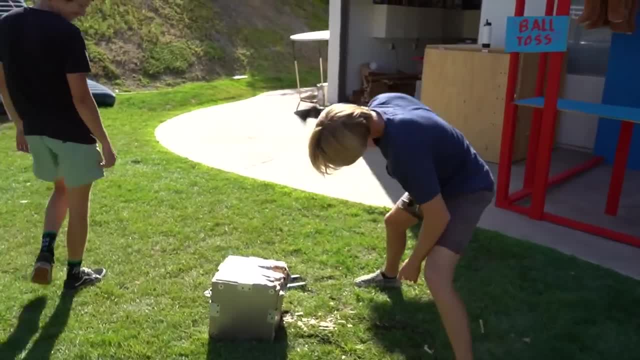 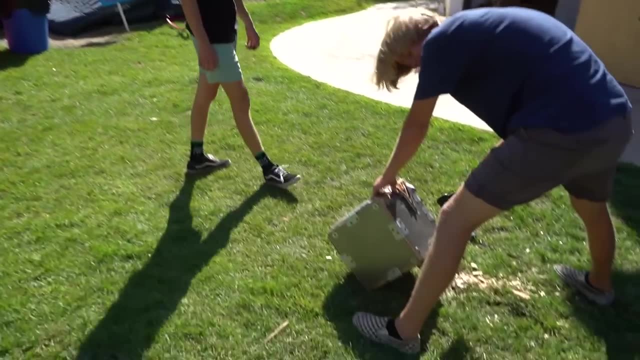 It's so light. Wait, I feel like Robert Knob, It's almost open. Look at this big hole, Ryan Dang. Look at this big hole I made. It's almost open. Look at this big hole, Ryan Dang. Look at this big hole I made. 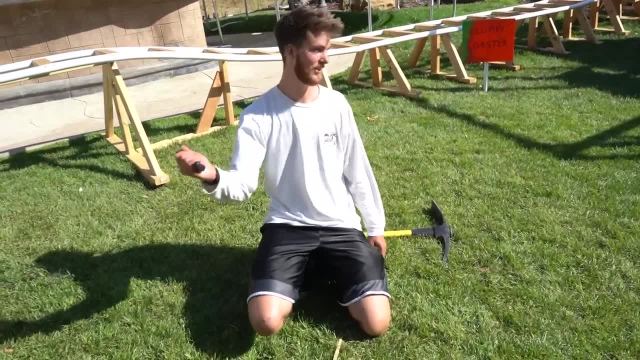 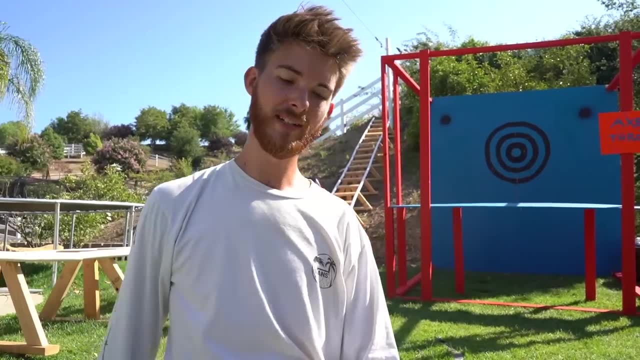 Dang, I just got to make it a little bigger. You know what I give up with this stupid. Now Chris is rendered useless and Jeffrey has the advantage. The weapon that I need is the mallet, Because it's small, I can target whatever I want. I'm not going to break my phone. 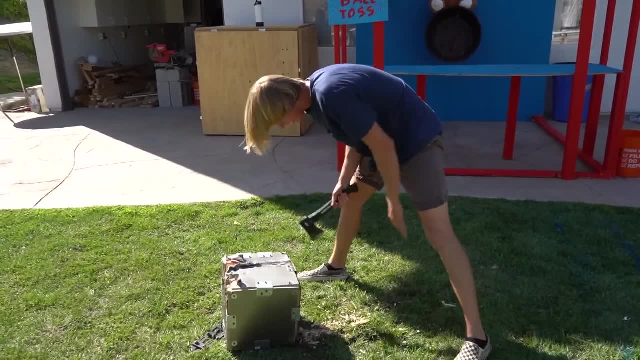 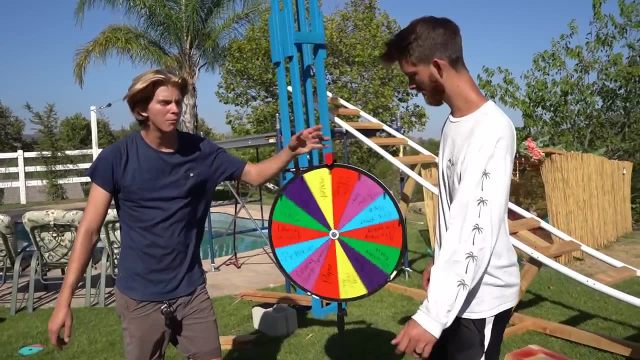 So hopefully I get that one. I made a crack all the way through the side. I think it's going to smash it open. Time to re-spin. Let's go to the board. Jeff, are you getting serious? Are you getting fired up inside your heart? 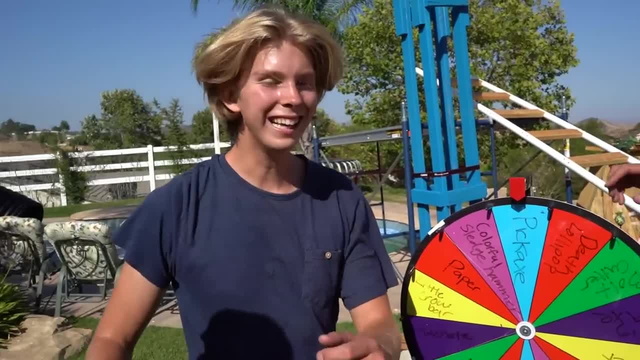 I'm getting fired up Pickaxe. Okay, dude, That's actually really good. I think I'm going to be able to do it. I'm going to be able to get out right now. If I get the pry bar, I might be able to get out too. 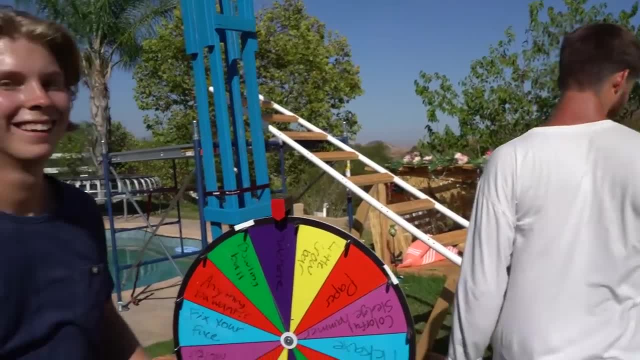 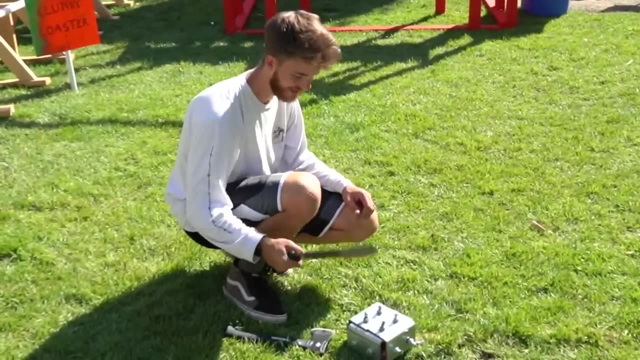 Don't get the pry bar. Don't get the pry bar. Machete, Machete, Dang. Will Jeff be able to break out of my box this round? Back to this again. Oh, That's a lot of damage right there. I just need to do. I have an idea. 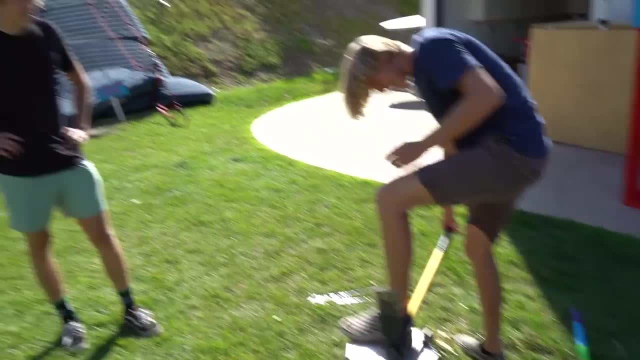 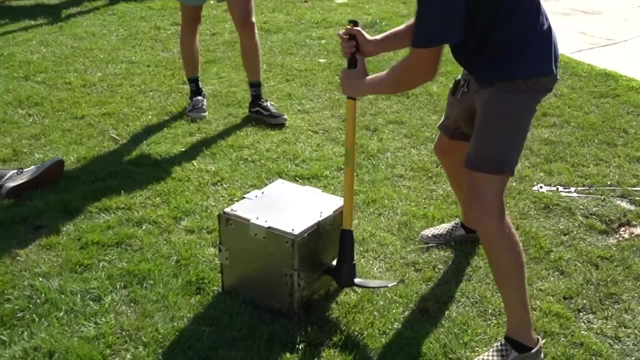 I need something to prevent it from moving upwards. I think Jeff got the pickaxe stuck. Did Jeff get the Jeff? Jeff, Come on, Dude. I heard your phone bounce around in there, bro. Axe throw more like machete throw. Oh my gosh, That's a surprise Bob. 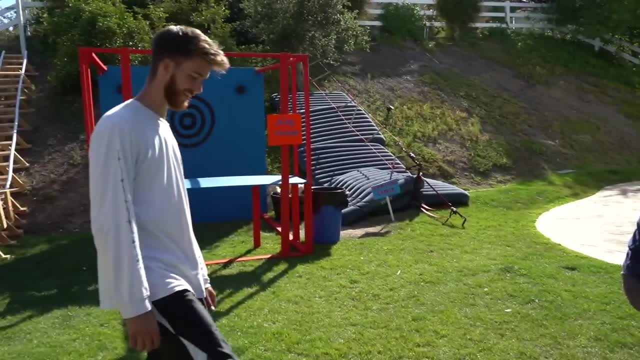 Your box is really strong. You got one more minute. Oh, Dude, I'm really widening this crack. I'm tired. guys, Give this video a like for encouragement to Jeff. Why not encouragement to me, Because you suck Dang dude? I can see my phone. 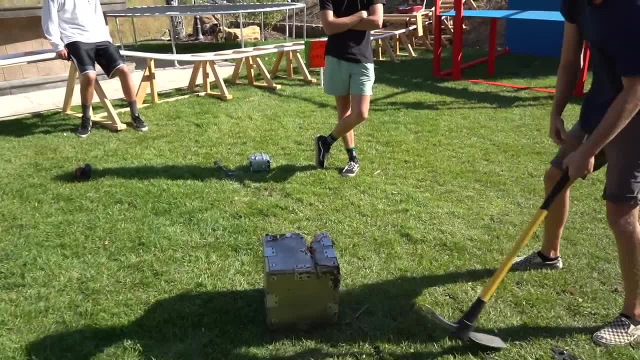 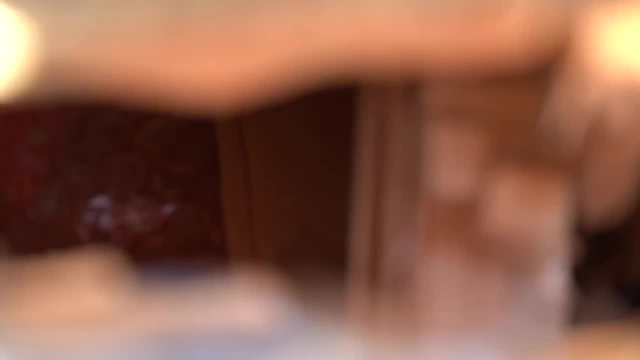 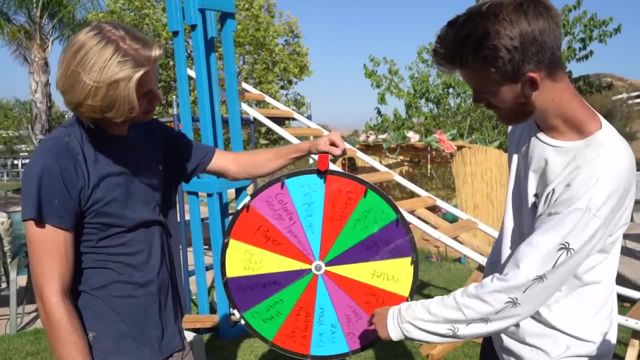 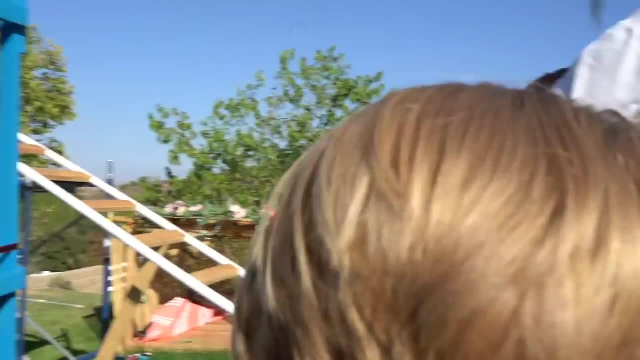 Big crowbars. Guess what I caught And purchased. Let me go. So what are all these cruising things? It says that you can keep all my big crowbars. Oh, it's a big crowbar. Or brands? I make 270 Purple, Purple, Machete. Alright, Heck this. 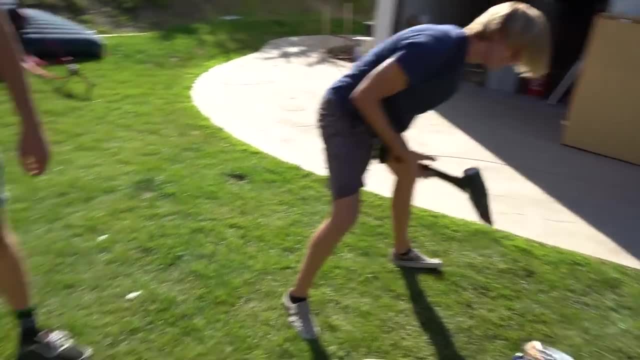 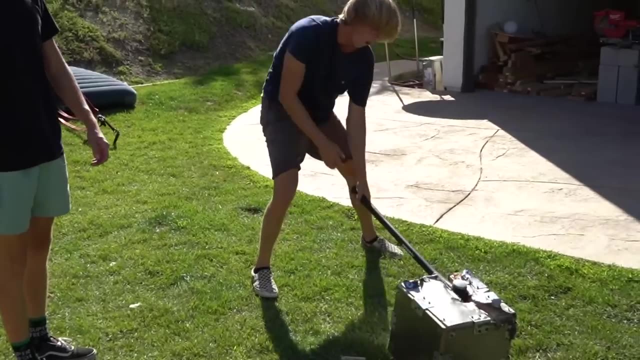 Pick whatever you want. Oh really, Dude, you better go quick. Wait, Where's the big crowbar? It's over there. Shoot. Oh dude, There's screws on the bottom. Come on, It's a race against time. Come on, There's screws coming out. Jeff might have just got it. 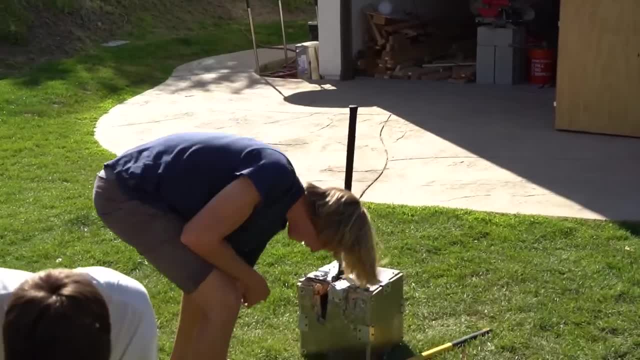 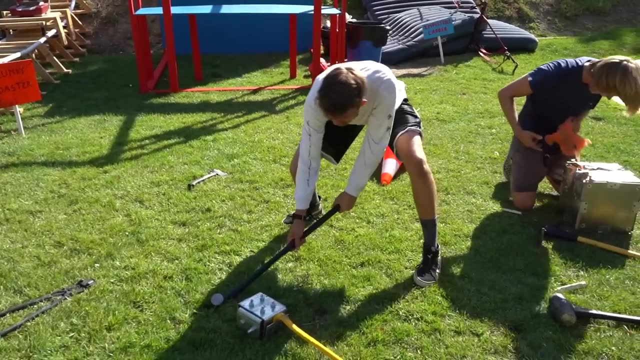 Jeff might have just got it. Come on, Oh, this is crazy, bro. Well, Jeff, be able to grab his phone. There's one piece of wood in the way, But I didn't get it out of the way. Yes, I got it. Oh, you got it. I got my phone. 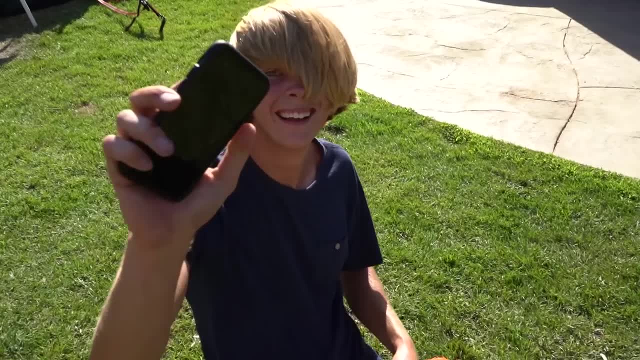 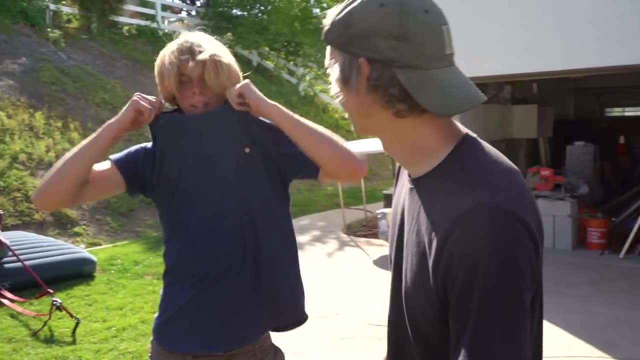 I'm pretty sure it's completely unharmed. Oh yeah, it's perfectly fine. Dude, Chris is the loser Apocalypse weapon I officially dumpster. I'm going to reward myself. Oh, it's a jumping in the pool. Just go to the pool. 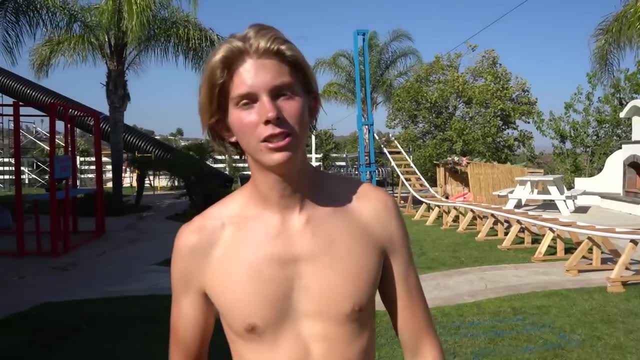 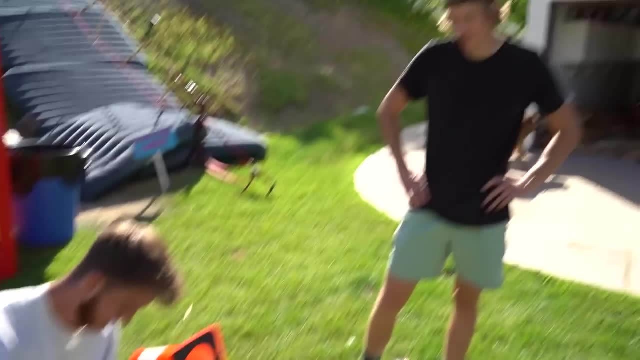 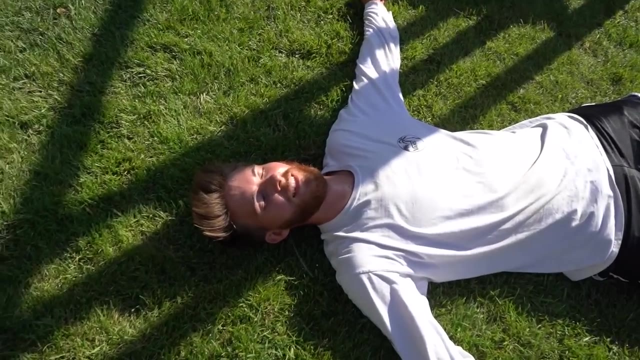 It's so hot Guys. so that means my box is the strongest, most unbreakable. I think we actually successfully created unbreakable box. So games over, bro, Let it go. It is over, Chris, Give up. This is being tossed in the trailer. It's over, bro. Huh, We're gonna have a. 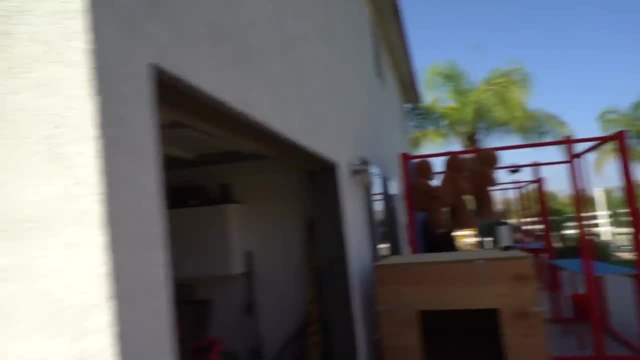 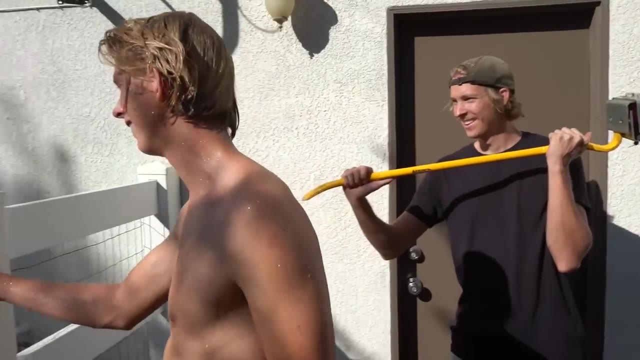 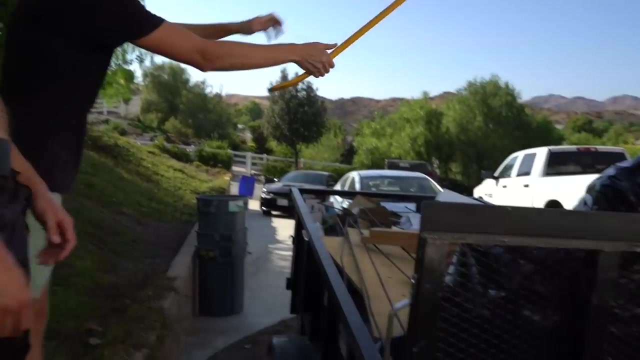 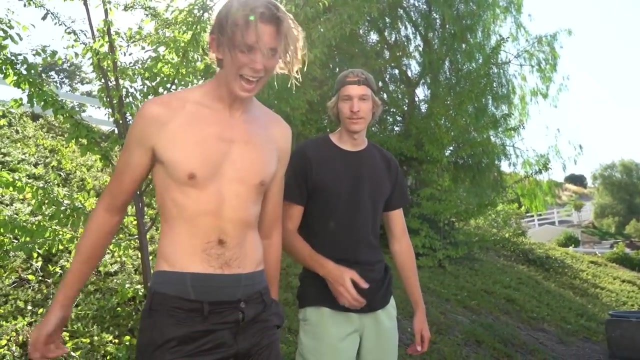 Ceremony. we need a funeral. you guys. that felt really good. victory feels sweet. Well, Jeff, it's not quite victory, cuz I won. This is the ultimate punishment right now. I hereby decree: Chris's phone is banished to the to the chamber. Robert, it's been a video, Jeffrey, guys.